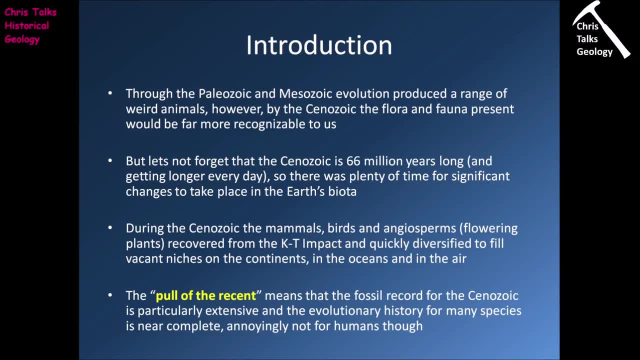 day. So this means that because there's a shorter time period, it means there's less chance for the fossil to be destroyed and lost from the fossil record, And so this means we have more fossils of Cenozoic animals, and so obviously that means our fossil record and therefore our understanding. 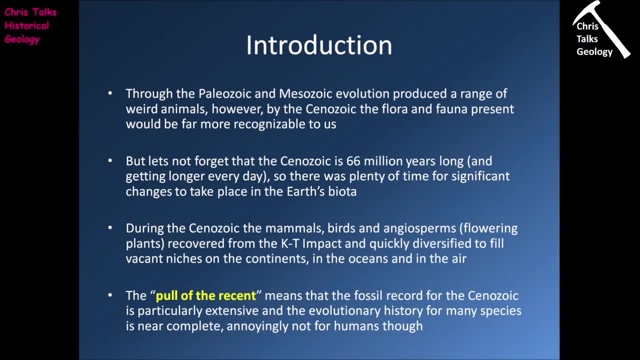 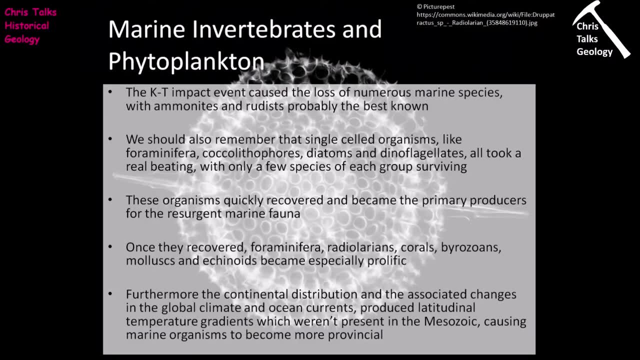 of Cenozoic evolution is going to be noticeably better when compared to the fossil record for the Mesozoic or the Paleozoic. Okay, so let's start in the oceans. So we're going to begin by thinking about marine invertebrates and phytoplankton, Now the Cretaceous-Tertiary. 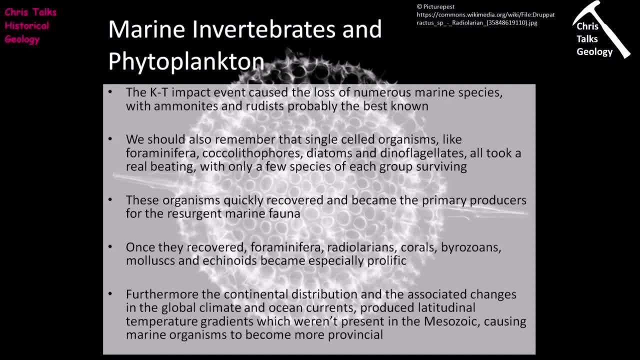 impact and the associated mass extinction caused the loss of numerous marine species, with, arguably, the ammonites and the rudis, probably the best known of the marine invertebrates that did not make it into the Cenozoic. Now, we should also remember that single-celled organisms like 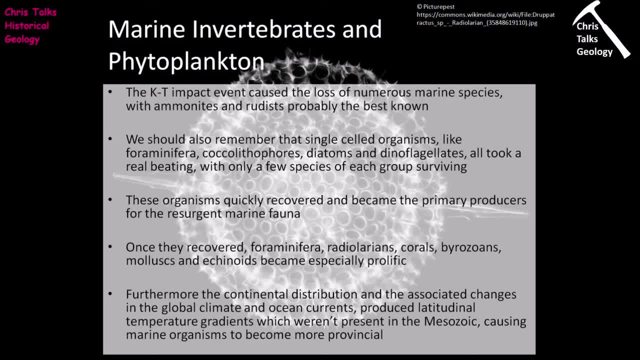 foraminifera, coccolithophores, diatoms and dinoflagellates all took a real beating during the Cretaceous-Tertiary mass extinction. However, a few species from each of these groups did manage to make it through into the Cenozoic. Now these species that managed to make it into the Cenozoic quickly recovered. 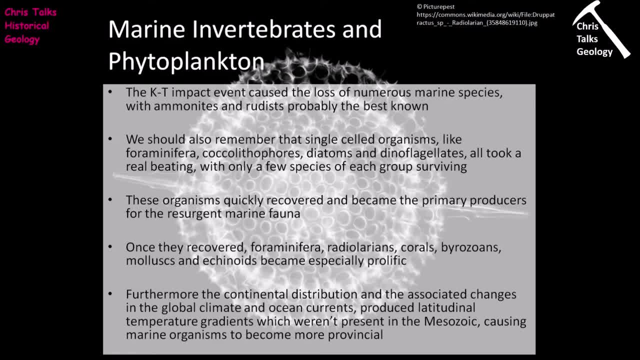 they diversified and they became the primary producers for the resurgent marine fauna. So their success essentially provides the primary food source to allow the marine environment to begin to recover. Now, in terms of the marine invertebrates, once they had recovered, groups like the foraminifera- 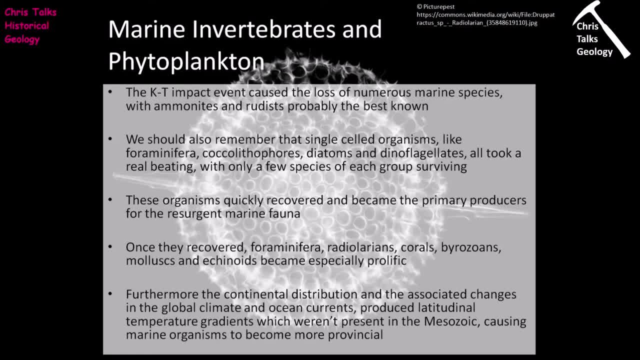 the radiolarians, the corals, the bryozoans, the mollusks and the echinoids all become particularly prolific during the Cenozoic. Furthermore, the continental distribution and the associated changes in the global climate and ocean currents produced as the continents move towards their 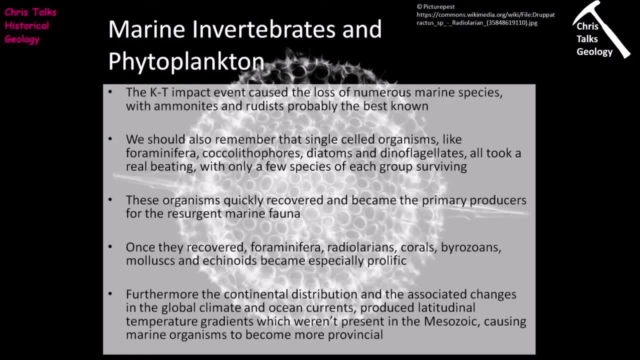 current positions led to latitudinal temperature gradients being established which weren't present in the Mesozoic. Now this means that each body of water that forms, so the North Atlantic, the South Atlantic, North Pacific, South Pacific, Indian Ocean, etc. is going to have its own. 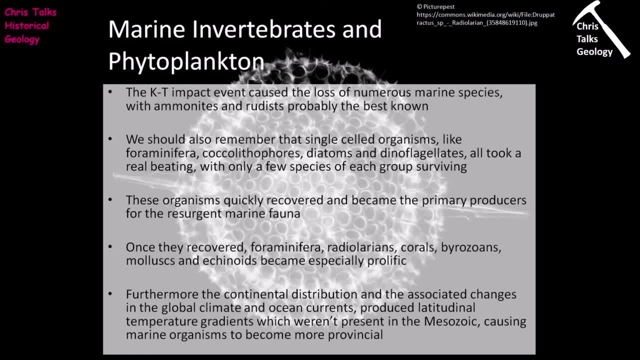 individual set of conditions, and so this is going to mean that life is going to adapt to those individual environments. So you're going to end up with a greater degree of diversity when it comes to marine fauna, and this is going to lead to organisms in general becoming more provincial. 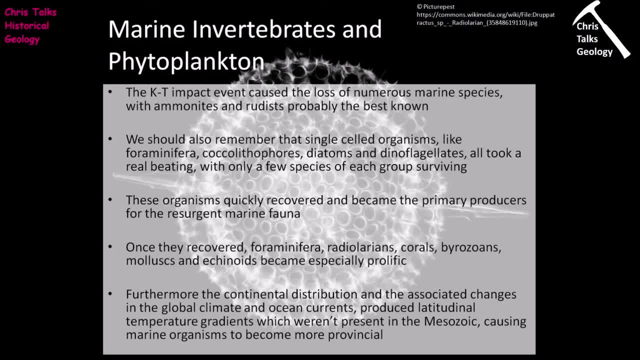 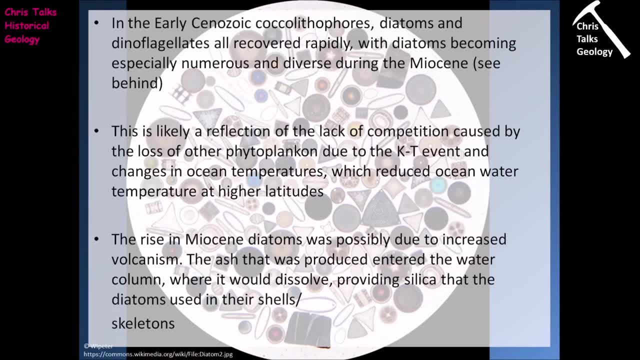 so they'll be more limited in their distribution. In the early Cenozoic we see the coccolithophores, the diatoms and the dinoflagellates all recover rapidly and this is going to be quite important because these single-celled photosynthesizing 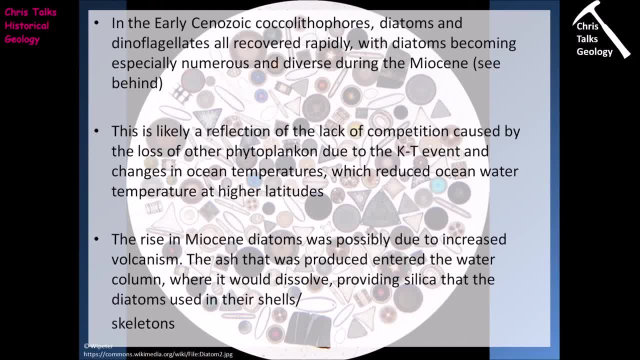 organisms that live in the water column are going to be very, very important because they are the basis of the marine food chain. Now. the diatoms in particular become especially numerous and diverse during the Miocene, so the increase in diatom diversity in numbers is likely a reflect. 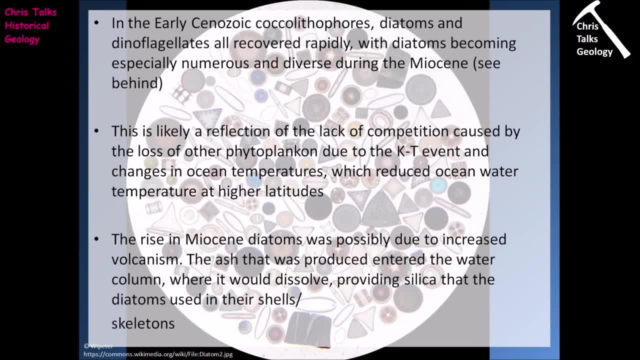 on the lack of competition caused by the loss of other phytoplankton. so there's simply less competition, more food, and so they begin to flourish. but there's also changes in ocean temperature which are advantageous for the diatoms. So, as we've discussed the temperature of the oceans, 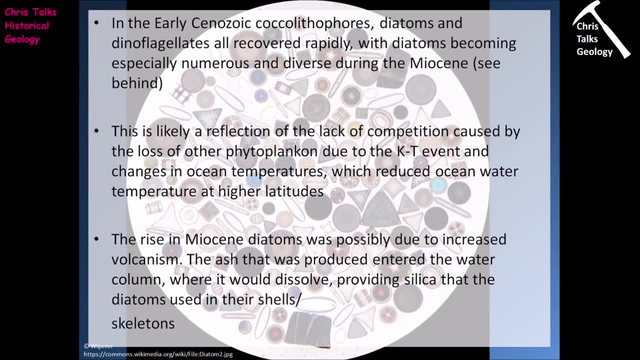 closer to the poles begins to decrease during the Cenozoic, and it just so happens that diatoms in particular, quite like cold water, and so, as we see these temperature changes occur, we begin to see diatoms becoming more and more established and more and more numerous in these colder water. 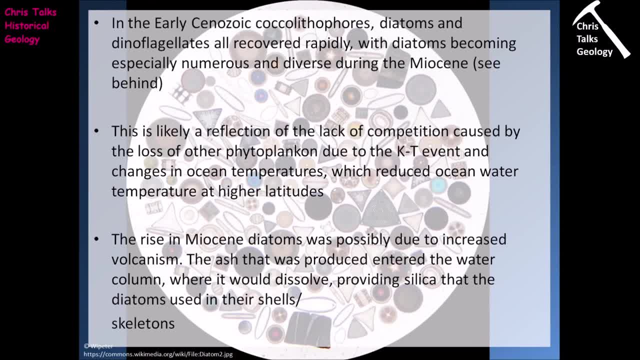 environments. Now, the rise of the Miocene diatoms is also possibly connected to increased volcanism, so one area in particular where we see diatoms doing extremely well is in the North Pacific, and this is an area that's going to be affected by numerous volcanic eruptions, particularly from 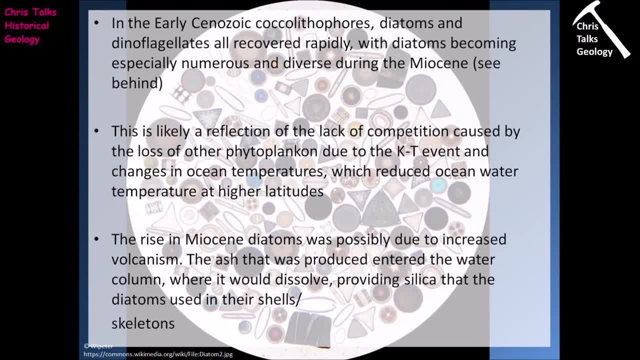 the Aleutian Islands, and so these explosive eruptions are going to put out large quantities of ash and dust, which is going to be thrown into the surrounding ocean. Some of this ash and dust will begin to dissolve into the sea water, so this will put silica, SiO2- into the sea water. 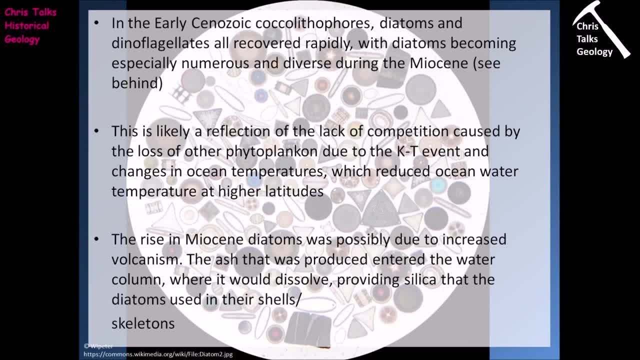 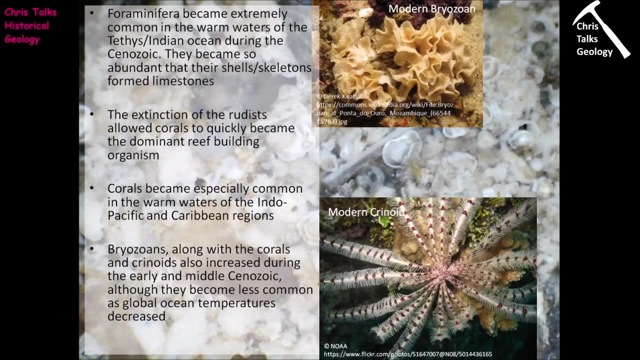 and this dissolved silica can then be used by the diatoms to grow their shells, and so the presence of this additional silica is going to be also quite advantageous for the diatoms. Another important marine microorganism are the foraminifera. Now, foraminifera are zooplankton. this means they do not photosynthesize. instead, they consume other 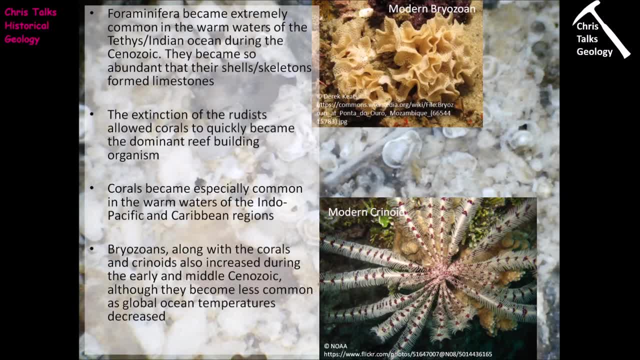 smaller microorganisms or food particles that they find on the sea floor or in the water column. Now, during the Cenozoic, we see foraminifera doing particularly well in warm water environments, with the Tethys slash Indian Ocean Basin a particularly hot spot for them. Now they 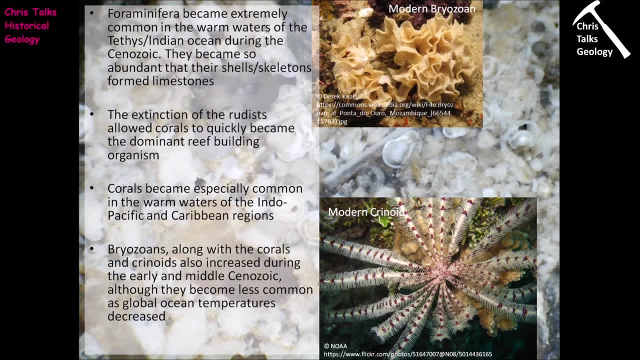 become so abundant in some cases that their shells slash skeletons will end up forming limestones. Now, just to give you some idea, foraminifera are microorganisms. they're tiny, so just try and imagine how many shells it would take to form a thick enough. 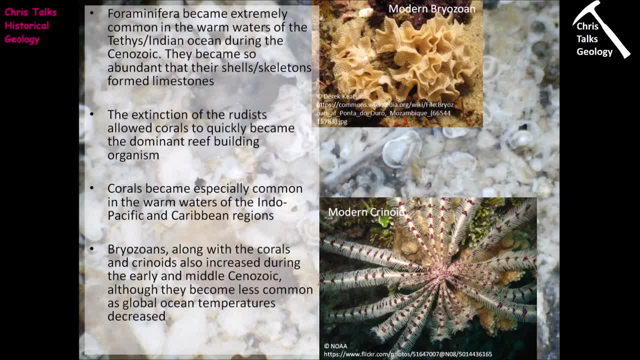 layer of sediment. to produce a decent sized layer of limestone. You would need literally billions or trillions of foraminifera shells in order to do this, so this shows you just how successful they are in these warm water environments during the Cenozoic. 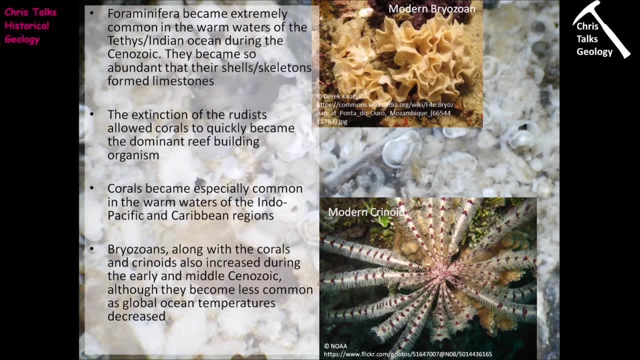 Now, in terms of reef building organisms, we know that reefs in the Mesozoic were dominated by the Rudists. Now the Rudists do not make it into the Cenozoic. they're killed off by the Cretaceous Tertiary Mass Extinction. Now this means in the Cenozoic the way is completely open for the corals. 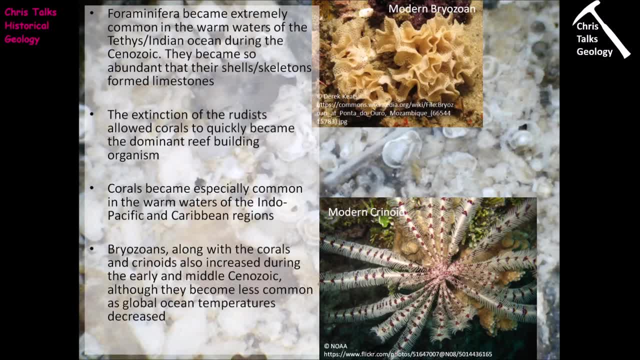 to become the dominant reef building organism. So what we see during the Cenozoic is we see the corals becoming especially common in the warm waters of the Indo-Pacific and the Caribbean and in this case, this is where we have the most common reefs around the Cenozoic. and, of course, 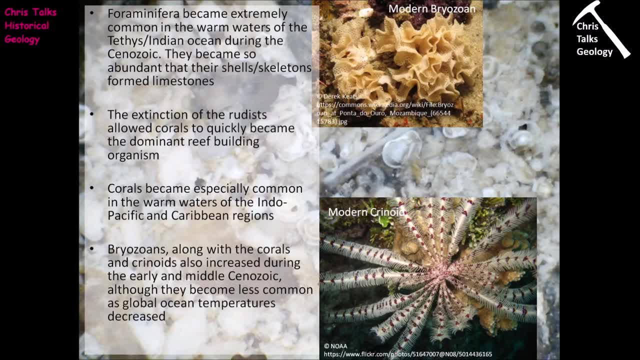 this makes perfect sense. these are the types of environments in which we would expect to find corals doing extremely well. Now, along with the corals, we also see bryozoans and crinoids increasing during the early to middle Cenozoic, so they are also important reef building organisms. 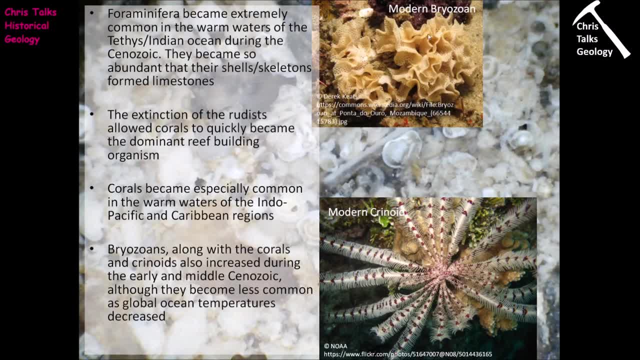 during the first half of the Cenozoic. Now, just to give you some idea, by the way, we have a picture of a modern bryozoan up here passes through these sieve-like structures and small food particles are removed and consumed. and here's an example of a fossilized Cenozerk bryozoan, just for comparison there. 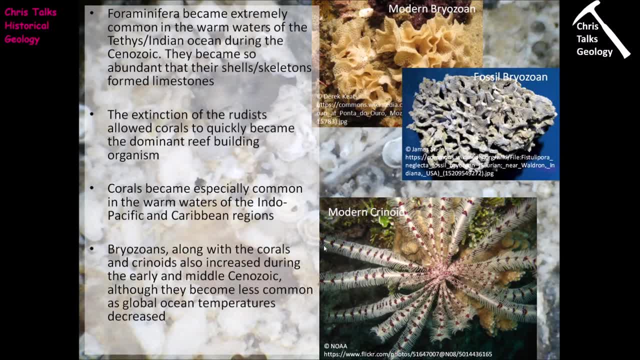 In terms of crinoids, they're also filter feeding organisms. they have these feather-like appendages on their limbs. they will catch small food particles which get passed down the limb to the base of the crinoid, down here where there's essentially a mouth, and behind the mouth obviously. 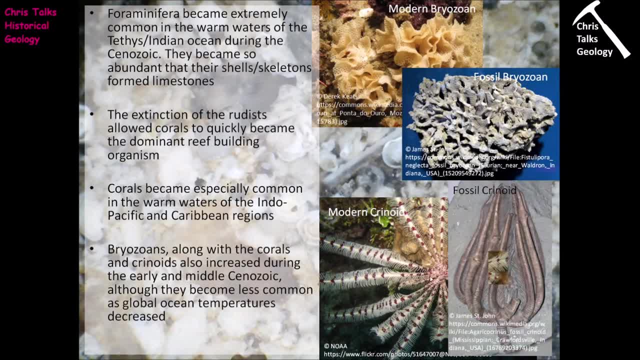 a stomach where the food particles will be consumed. and once again, here's a crinoid fossil, just to show you what they look like in the fossil record. Now, as I was saying, the bryozoans and the crinoids do pretty well in the early to middle Cenozerk, although we do see them becoming less. 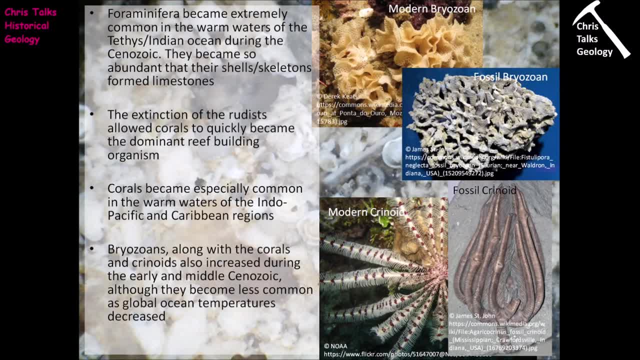 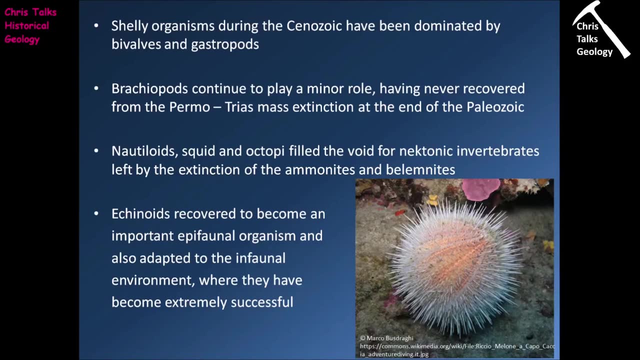 common as global ocean temperatures begin to decrease in the later portions of the Cenozerk. so although they are still important reef building organisms, they aren't as important as they were in the first half of the century. So in terms of the shelly marine invertebrates, we see that during the Cenozerk, the bivalves and 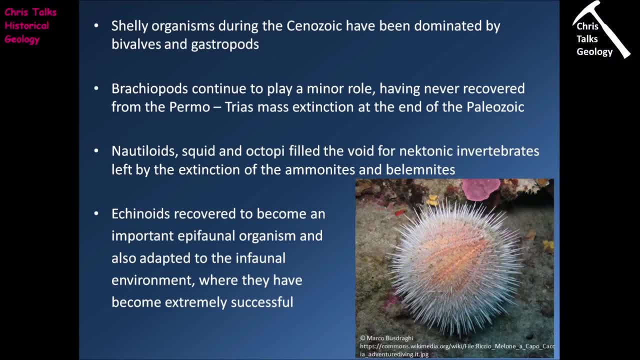 the gastropods become dominant. Now the brachiopods are also present, but they are a relatively minor component of the marine invertebrate faunas, and that's because they've never really recovered from the permotrius mass extinction at the end of the Paleozoic. From that point on they were 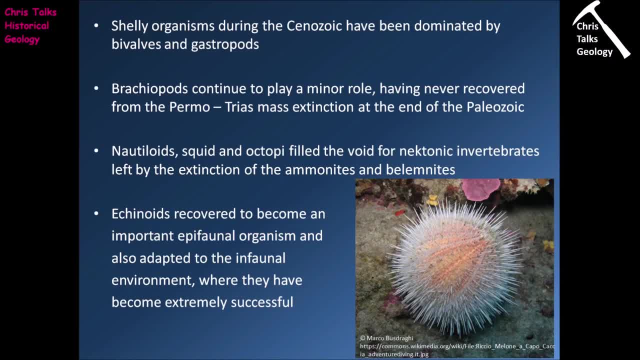 just being out-competed by the bivalves. all the way through the Mesozoic, And that's continued into the Cenozoic, We see nautiloids, squid and octopi fill the void for nectonic invertebrates left by the loss of the ammonites and the belemnites. So if you remember, 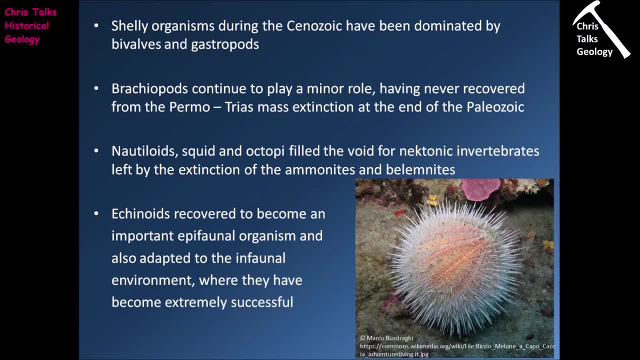 the ammonites in particular were very, very numerous in the water column during the Mesozoic. but of course, as we move into the Cenozoic, they are gone, and so we see the nautiloids, the squid and the octopi taking that niche. In terms of the echinoids, we see them recover and they become an 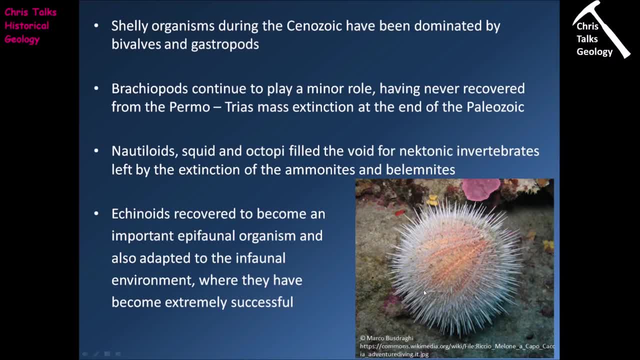 important epi-faunal organism. So we see lots and lots of, for instance, sea urchins moving across the seafloor. so that's the epi-faunal environment. We do, however, also see some of the echinoids making their way into the in-faunal environment, so actually going down into the sediment and once 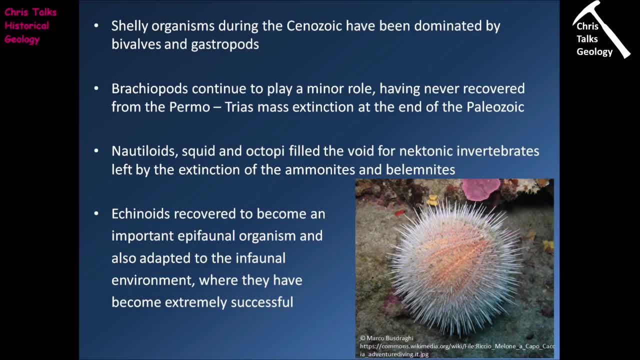 again. in this environment they become particularly successful And we can actually see this change quite nicely in the fossil record. So if we look at this sea urchin here, you'll notice it's covered in spines, obviously For defensive purposes. Now, if you're on the seafloor and you're exposed, having spines is a 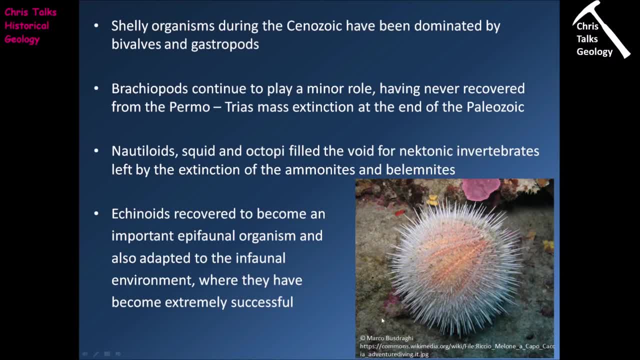 great idea. However, the second you try and move through, any sediment having spines actually becomes an impediment. They get in the way. So what we can see in the Cenozoic is we see the appearance of a number of relatively smooth shelled echinoids, and so this is showing us. 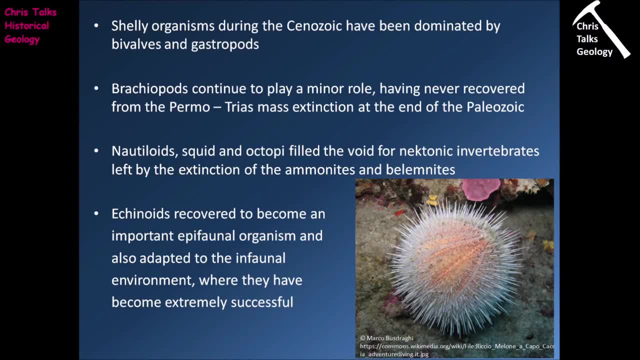 they're moving from the exposed epi-faunal environment into the more protected in-faunal environment. So some of you are probably wondering: okay, well, what was happening during the Cenozoic with regards to the marine vertebrates? Well, we know that the most advanced form of fish, the teleosts, were. 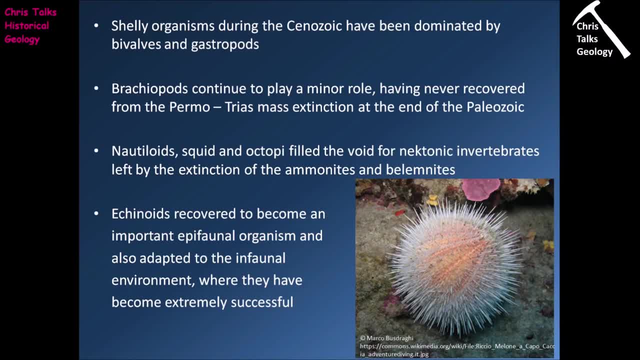 established in the Mesozoic and they make it across into the Cenozoic and they simply increase in number and diversify throughout the Cenozoic. The same goes for the cartilaginous fish. that includes the sharks. So when it really comes down to it, there aren't significant changes. 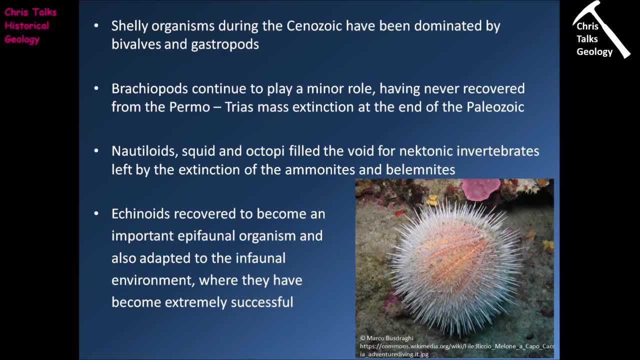 when it comes to the fish that are in the Cenozoic. So we can see that the fish that are in the Cenozoic are moving towards the marine vertebrates. Now, the one major change that does occur is that from the mid to late Cenozoic we are going to see the introduction of large amounts of marine 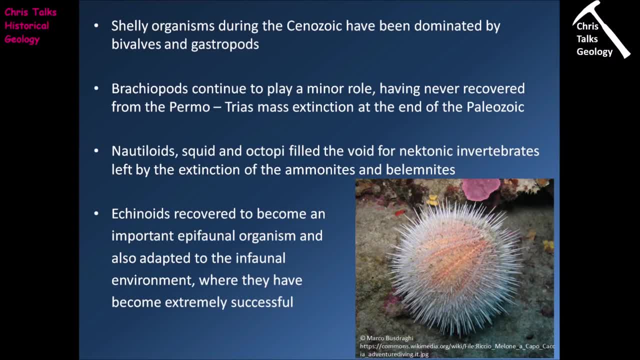 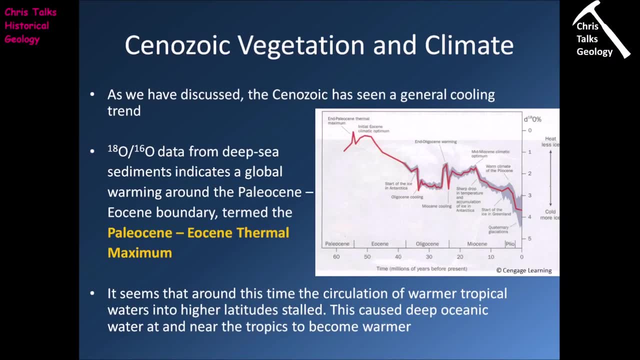 mammals, in the form of whales and dolphins, for instance, and we're going to be discussing those in greater detail later in this presentation. So now let's move on to Cenozoic vegetation and climate. Now, as we've discussed in the past, the Cenozoic has seen a general cooling trend and 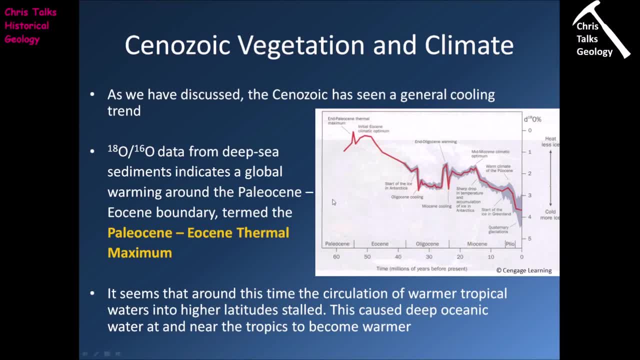 we can see it on this diagram over here. We've seen this diagram before so I'm not going to discuss it. but what you can see is over time there's been a gradual decrease in temperature during the Cenozoic. We can see that decrease in temperature hasn't been a smooth, gradual change. 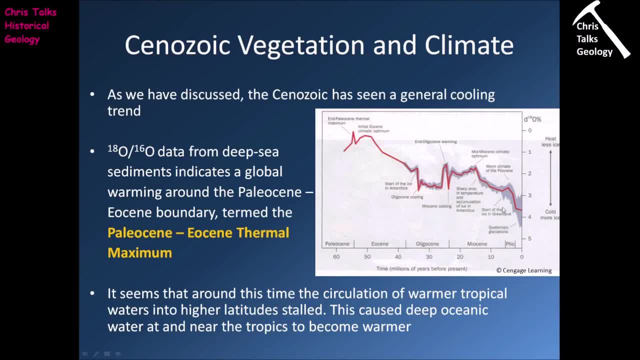 it's been. it's had quite a lot of topography, but on the whole we can see the downward trend is quite clear. Now, oxygen 18: oxygen 16- data from deep marine sediments indicates that there was a global warming period around the period of the Cenozoic. So we can see that there's been a gradual decrease in. 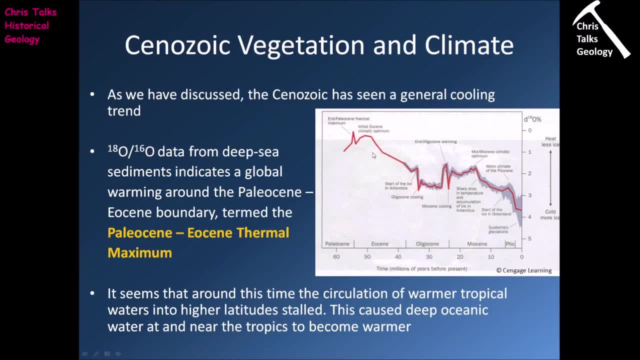 temperature. If you look at this diagram, the Cenozoic is also showing a very typical warming period during the Cenozoic. This is very clear because it shows that it's the Palaeocene-Eocene boundary. So this region right here and this is referred to as the Palaeocene. 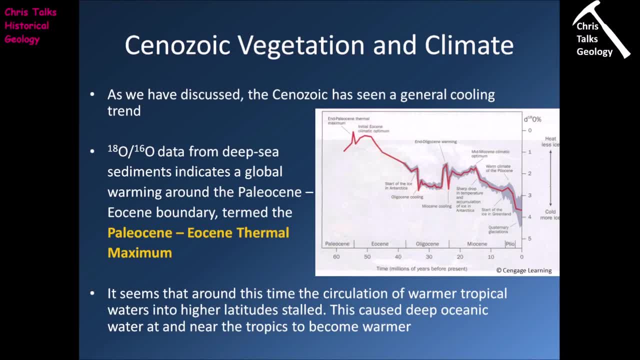 thermal maximum. This is when we're going to have the highest temperatures occurring during the Cenozoic. Now it seems that around this time the circulation of warmer tropical waters into the higher latitudes stalls, and this results in deep oceanic water at or near the tropics becoming 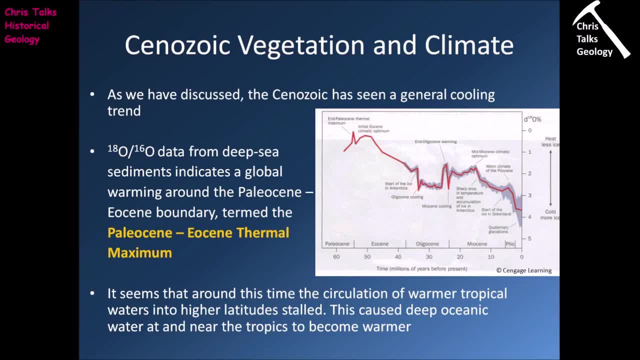 warmer. So typically what happens is we've got a lot of heat coming in from the top, of the water gets warmed up in the tropics and then it moves towards the north or the south pole, and as this warm water leaves the tropics, it gets replaced by cold water being pulled in along the sea floor. 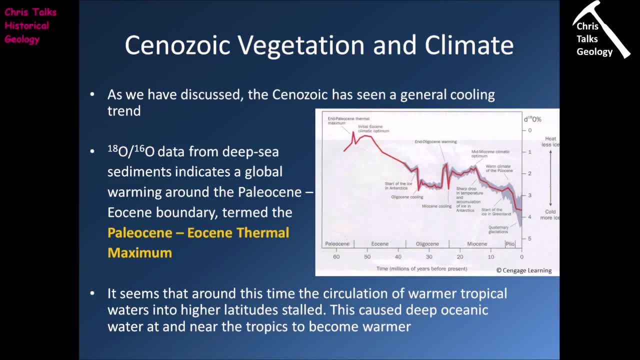 from the higher latitudes towards the equator. so essentially we have a conveyor belt system. warm water moves towards the poles and colder water from the poles gets pulled back down towards the equator. so we have water constantly being replenished. now what we see happening in the 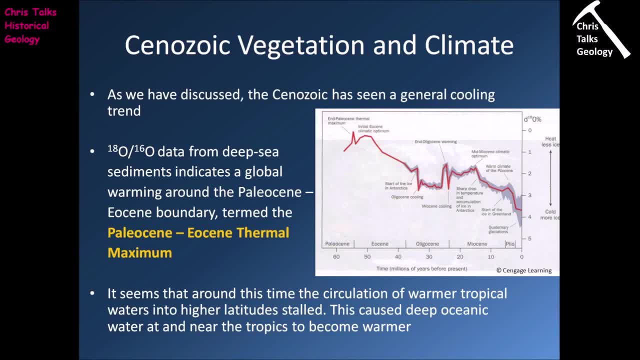 cenozoic is for a period of time, especially around this paleocene eocene thermal maximum, we think this circulation begins to stall a bit, and so what this means is you're not having cold water coming back into these equatorial regions, and so we begin to see the the water temperature. 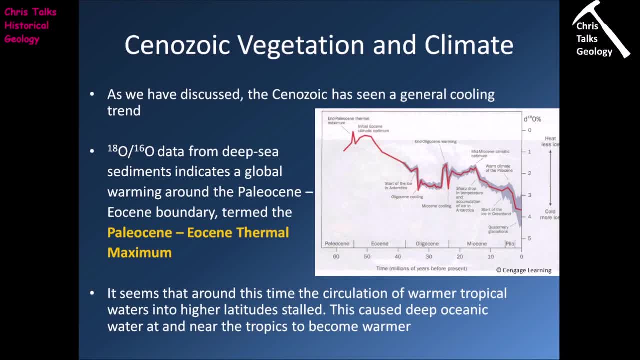 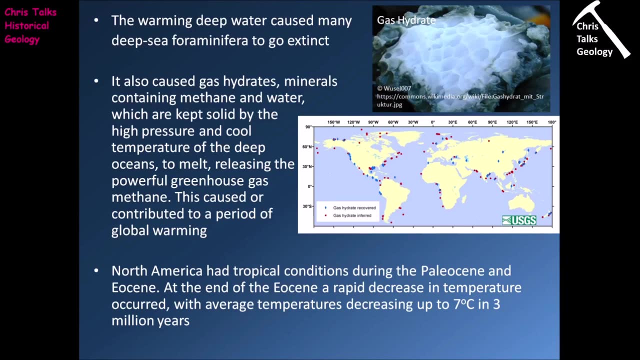 in these equatorial regions becoming warmer and warmer, both on the surface and in the deep marine environment, so near the sea floor, and this is going to become very, very important. so you I'm going to show you a picture of a gas hydrate. so a gas hydrate is a mixture of methane and water. 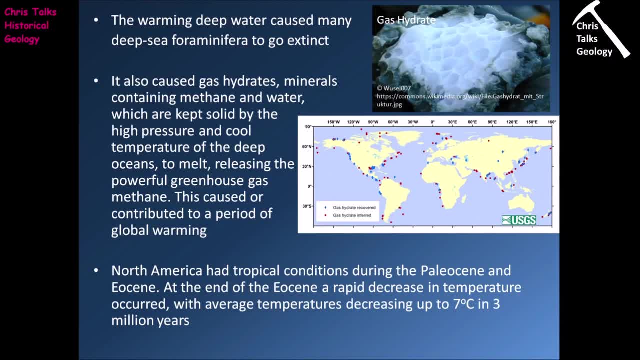 which is put under lots and lots of pressure at quite low temperatures, and it causes the methane in the water to form a solid phase, which we call gas hydrate. now the problem is is that gas hydrates are just extremelyeb. Venice beautiful gas, is it? it's too well melts, too disagreeable versus very 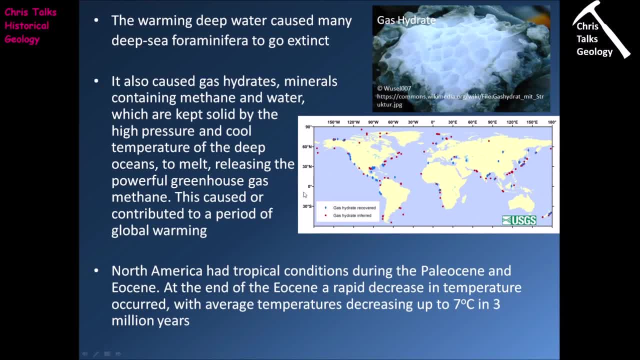 like warm temperatures. so the second, the deep ocean water in these equatorial regions began to warm up. well, that's going to cause the gas hydrates to become unstable, and so this is going to mean they're going to break down in the methane in them is going to be released, and that meet. 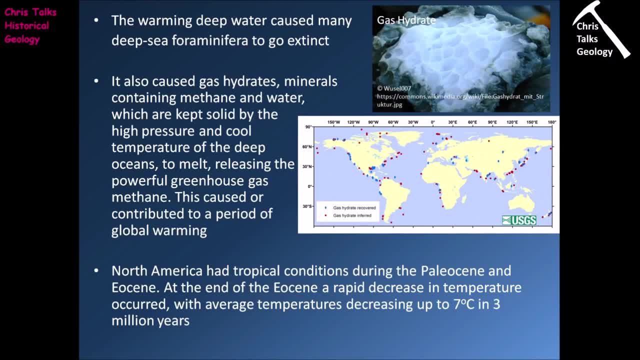 them obviously bubble up from the sea floor and into the atmosphere and, as we know me, breathe I very strong greenhouse gases, about 20 times more powerful than carbon dioxide, and so a large release, a large release of methane produced by gas hydrate destruction, will cause a very substantial change. 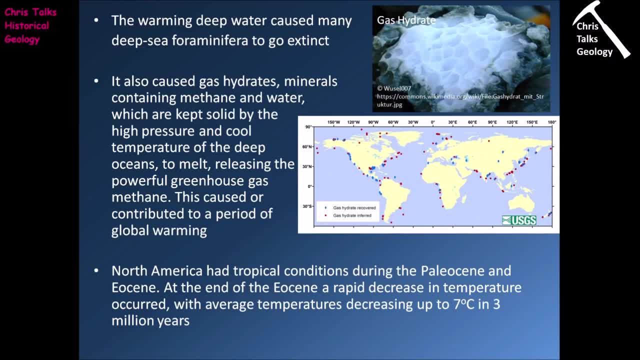 in the greenhouse effect, leading to a period of global warming, And this is what we're probably seeing at this Paleocene-Eocene thermal maximum. Now, in terms of North America, we can see that we have tropical conditions during the Paleocene and the Eocene during this period of high. 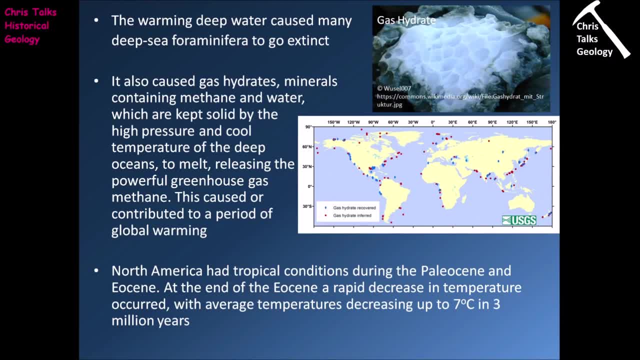 temperatures. Now, at the end of the Eocene, we begin to see a rapid decrease in temperature, with average temperatures decreasing by up to 7 Celsius in a period of about 3 million years. So as the Eocene is coming to the end and we're heading into the Oligocene, something is clearly: 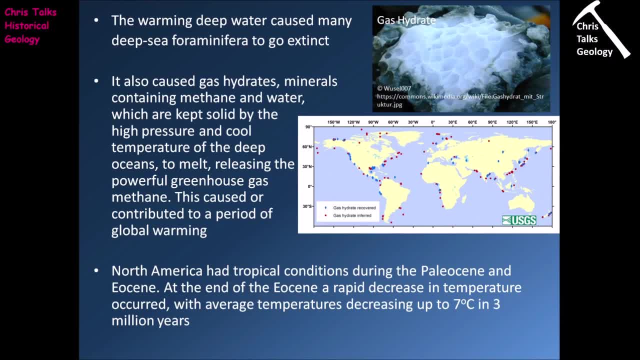 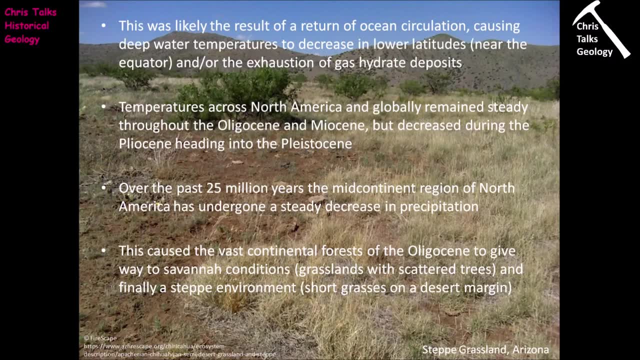 changing. that's causing the greenhouse effect to become weaker. So there are a couple of possible explanations which might explain the weakening of the greenhouse effect that we see at the Paleocene and the Eocene. So let's take a look at some of the explanations that we see at the 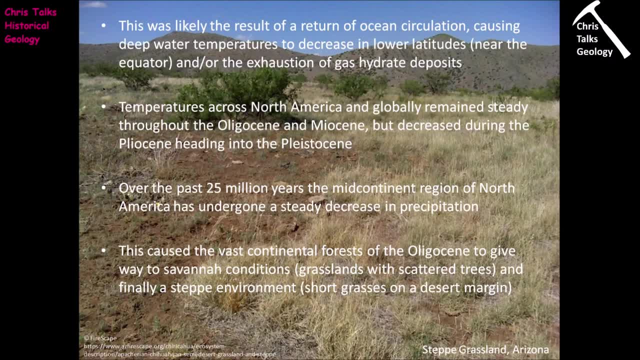 end of the Eocene. The first possibility is that we re-establish ocean circulation Now. this is going to allow colder water from higher latitude environments to begin to move back towards the equator, So this means that these deep marine tropical environments that were experiencing 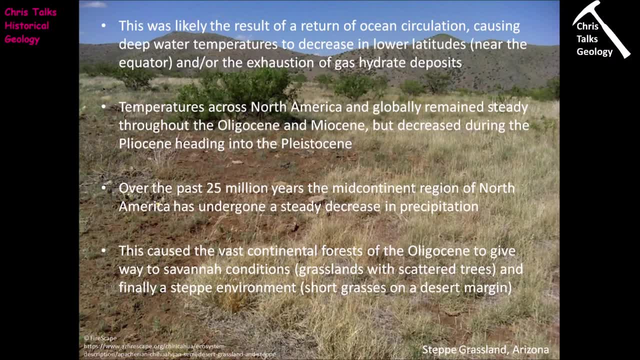 elevated temperatures are all of a sudden going to have an influx of cold water And this is going to help to drive down the water temperature and stabilize any gas hydrates that are still present. Obviously, once the gas hydrates are stabilized, they're going to stop breaking down and releasing. 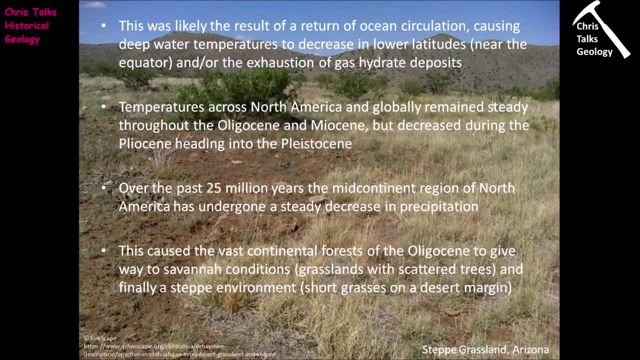 methane. The other possibility is that maybe by the end of the Eocene, the tropical gas hydrate deposits have simply been exhausted, So there's no more gas hydrate actually left to break down, And if there's no more gas hydrate, that means no more methane being released. This means any 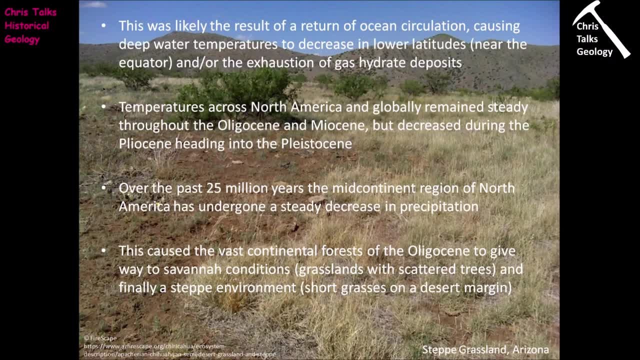 methane that's present in the atmosphere towards the end of the Eocene will steadily be stripped out, And so, over time, we're going to have an influx of cold water, And so we're going to have to see a steady weakening of the greenhouse effect and therefore a decrease in global 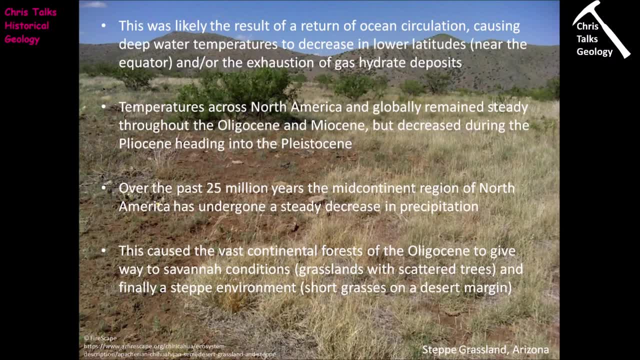 temperatures. Now, as we transition from the Eocene into the Oligocene, we do see that global temperatures drop And we see the Oligocene on the whole has relatively stable conditions And this affects both the North America and globally. So on the whole, during the Oligocene everything 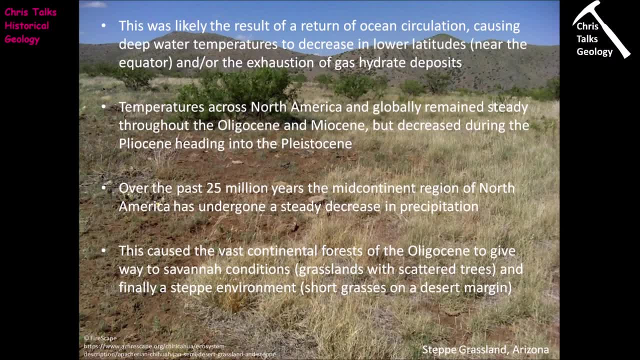 is pretty stable. Now, as we head from the Oligocene into the Miocene, there is a bit of a temperature spike. However, by the end of the Eocene we're going to see a steady weakening of the temperature. By the middle Miocene this spike has essentially evened out, And so, when we look, 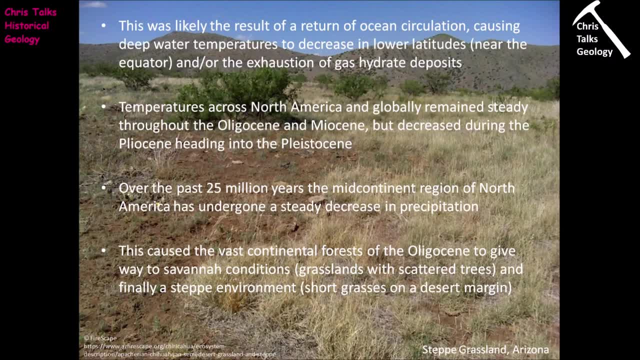 at the Oligocene and Miocene as a whole, we see that in general, if we average it out, the temperature is relatively stable. Now, from the middle Miocene onwards- so that's heading into the Pliocene and the Pleistocene- we see that there is a noticeable and quite sharp decrease in global temperatures. 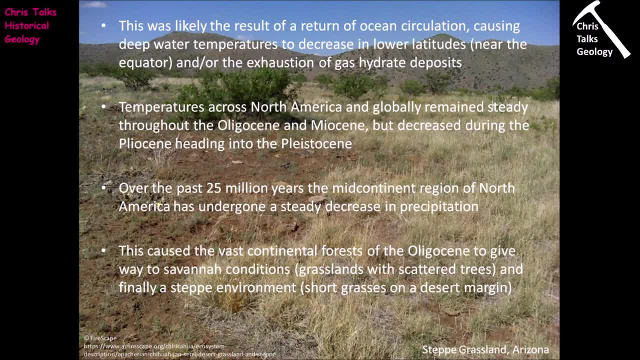 Now, over the past 25 million years, so that's from the middle Miocene until the present day, we've noticed that the mid-continent region of North America has undergone a steady decrease in precipitation, And this is associated with this general decrease in global temperatures. 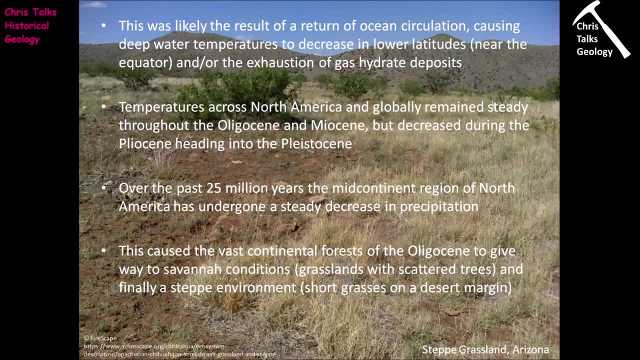 So this change in the global environment caused the large Oligocene forests, which did cover the centre of North America, to begin to die back and they are replaced by savannah conditions. So savannah conditions essentially means you have lots and lots of grasslands. 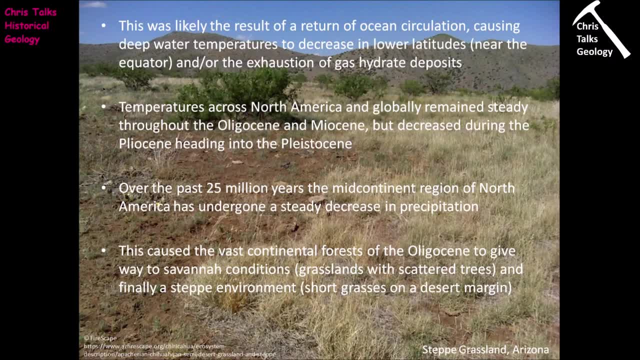 with scattered trees, and so this is reflecting both a decrease in temperature and also a decrease in precipitation. so conditions are getting harder, and the forests of the Oligocene begin to die. back now, as this temperature decrease begins to accelerate, we begin to see even the savannah. 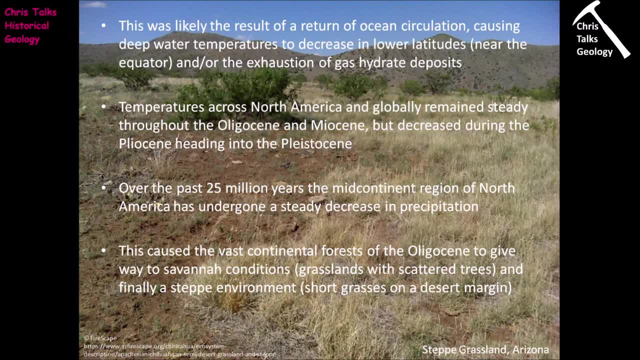 conditions begin to become untenable and the savannah organisms begin to get replaced by step by step environment, and so, in a step environment, we start to see the introduction of short drought resistant grasses, and so this is the type of environment you tend to get forming. 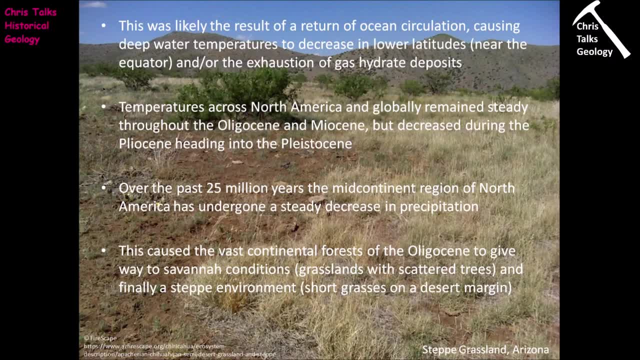 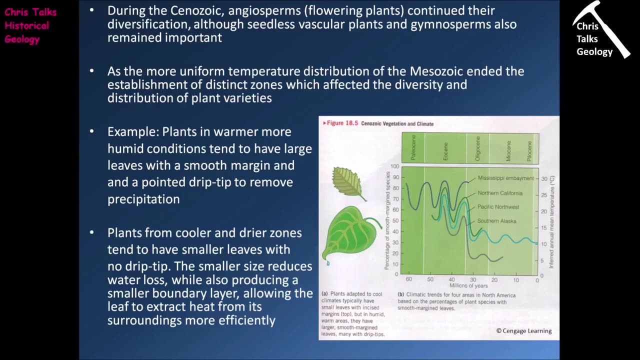 along desert margins, and so this change in the fauna and flora of the interior of North America is reflecting this general cooling trend we see from the middle Miocene onwards, so during the Cenozoic. we see the angiosperms, that's the flowering plants, continue their 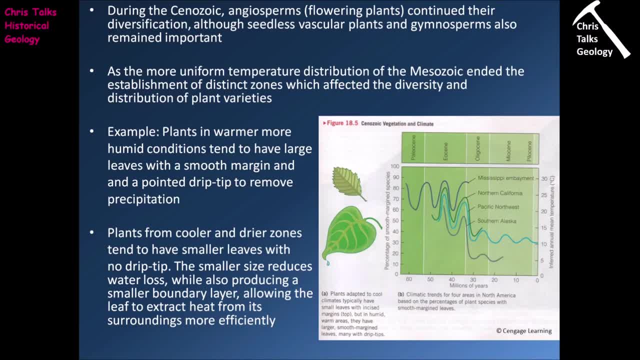 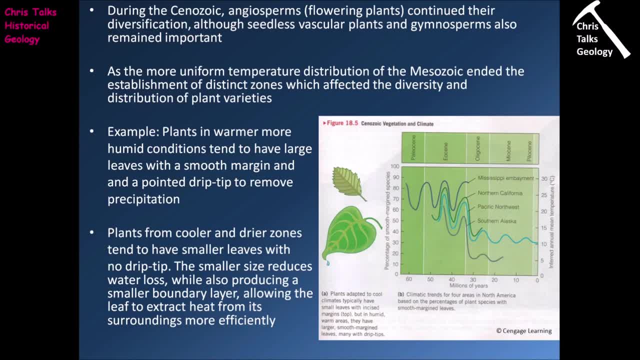 make it through the Cretaceous tertiary mass extinction and they very quickly re-establish themselves and continue their dominance over the seedless vascular plants and the gymnosperms. now, the seedless vascular plants and the gymnosperms are still important groups of plants. however, their distribution is far more limited, so we've already discussed how seedless 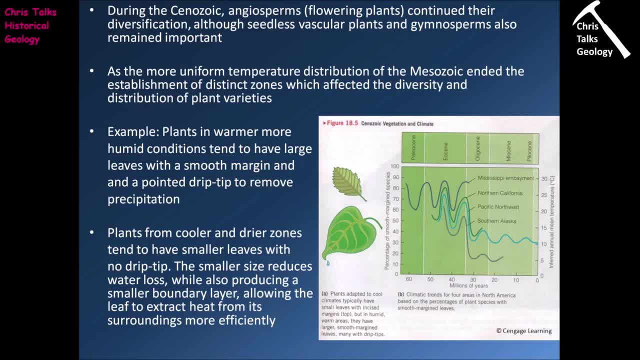 vascular plants are, on the whole, limited to environments which tend to be quite wet, whereas the gymnosperms are typically limited to environments which are now quite cold and dry. so think of environments like the coniferous forests of Northern Canada and Northern Russia. so as we transition into the Cenozoic, we see the loss of the uniform temperature. 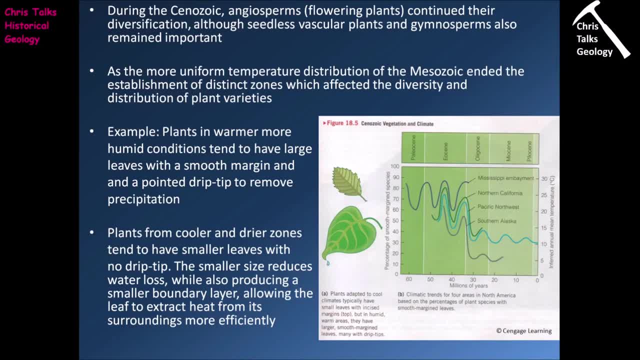 distribution which we experienced during the Mesozoic. so, if you remember, during the Triassic, Jurassic and Cretaceous we had a more homogeneous atmosphere and this meant that warm weather conditions extended quite a long way north and south from the equator. so just to give you some idea, we were experiencing conditions. 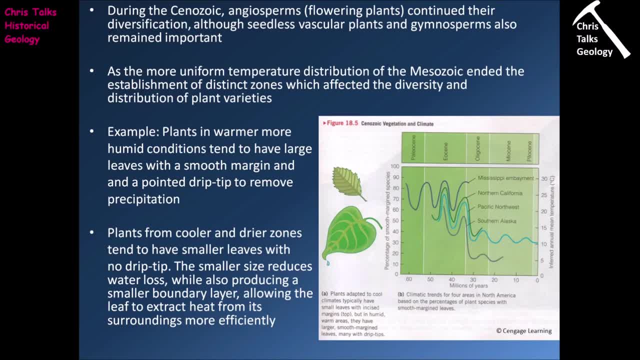 which could be described as temperate to tropical, all the way as high as 60 degrees north of the equator, that's the southern tip of Greenland. now, this means that because you had this, you know- nice homogenized environment, it meant that plant life that was comfortable existing in the tropics could 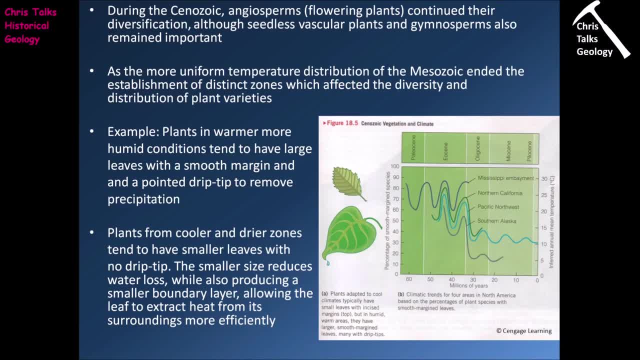 extend quite a long way north or south of the equator, and this resulted in quite a homogenous makeup when it came to flora during the Triassic, Jurassic and Cretaceous, because they could be so widely distributed, because the conditions were so similar. now, as we move into the Cenozoic, we see the establishment of 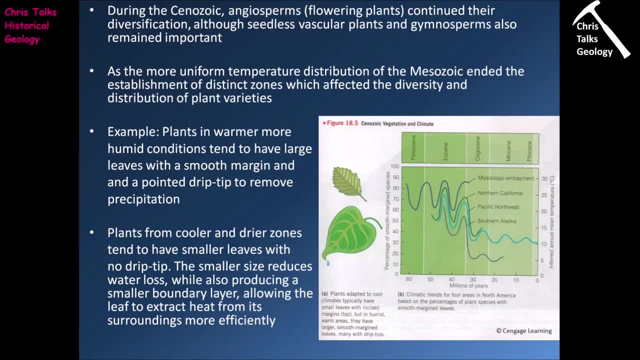 distinct climatic zones, and obviously each of these zones is going to have its own set of conditions, and so this is going to mean plants are going to have to evolve to meet those conditions. so we're going to see an increase in the diversification of plant life and we're going 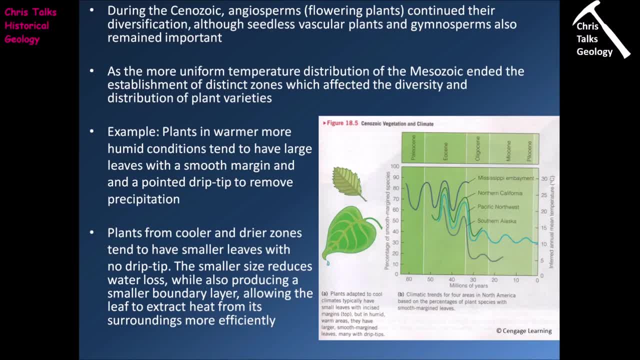 to see plants become more limited in their distribution because they become so specialized to those specific conditions. now a good example of these specializations is the leaf design shown by plants from warm, humid climate. so think of something like a rainforest now. these leaves tend to have quite a large size. they tend to 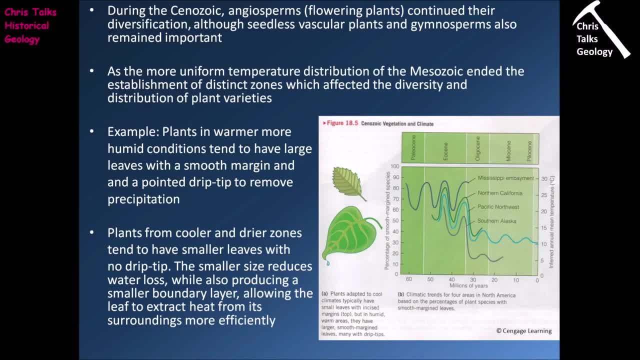 have smooth margins and they tend to have what's referred to as a drip tip. now, the size of the leaf is a reflection of the fact they are living in an environment which is very, very wet, and typically the larger the leaf, the more water you will lose through the process of transpiration. 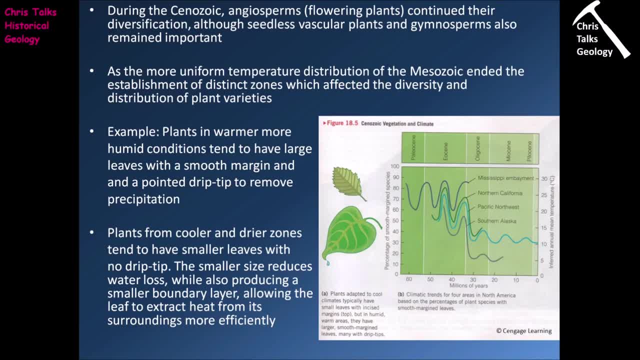 so think of that essentially as the plant sweating, so larger the leaf, the more water you will lose. however, because these plants are living in an environment that has a very, very high rate of rainfall, it means they can very quickly replace any water which is lost, and so this means they have the capacity to have quite large leaves, and this is advantageous. 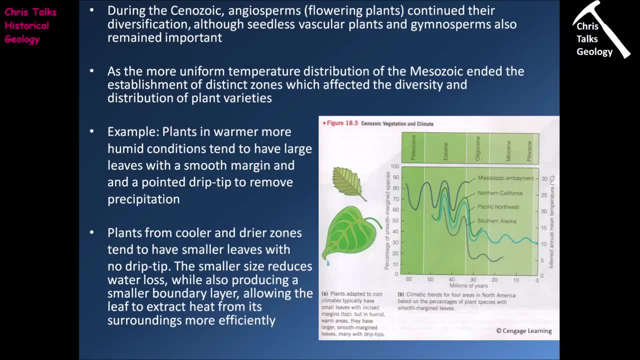 because the larger the leaf, the more sunlight it can collect and so the more efficient you be at photosynthesis. now in terms of the other leaf, other portions of the leaf, design, the smooth margins and the drip tip. this is a design feature that's required to get water off the leaf as fast. 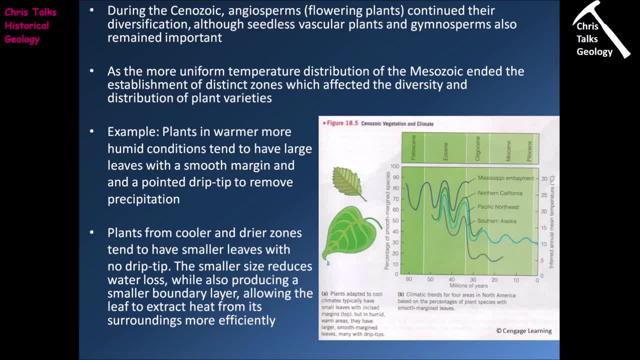 as possible. so having water sitting on your leaf is actually going to inhibit your ability to successfully photosynthesize. so what you want as a plant is you want to get that water off your leaf as fast as possible, and so having the smooth margins and the drip tip helps these leaves to 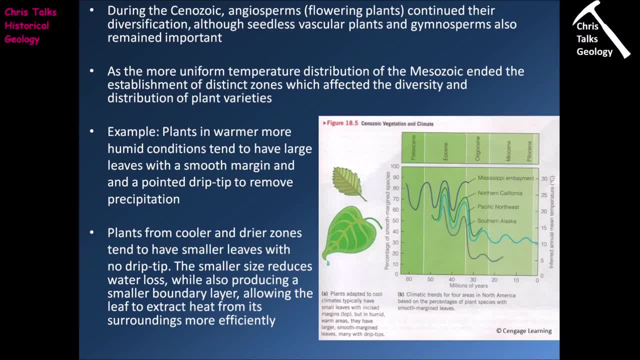 get rid of the water off the surface, thereby allowing them to photosynthesize at the heart, you know, with greatest efficiency. when we look at plants from cooler, drier zones, we see they tend to have smaller leaves and no drip tip. now, when i'm talking about a cooler or drier zone, i'm talking 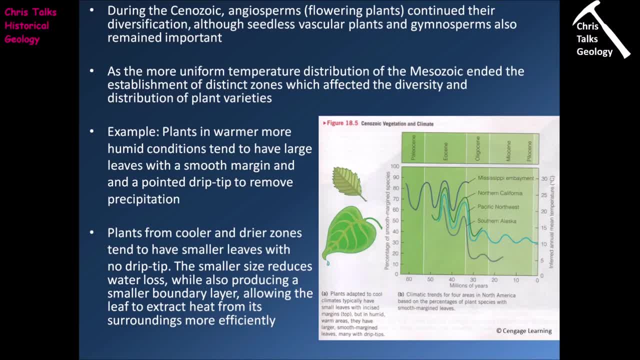 about a more temperate environment, similar to the type of environment experienced by much of north america and europe. now, the smaller size reduces water loss. so, as we've already discussed, the larger the leaf, the more it's going to be able to get rid of the water off the surface. so, 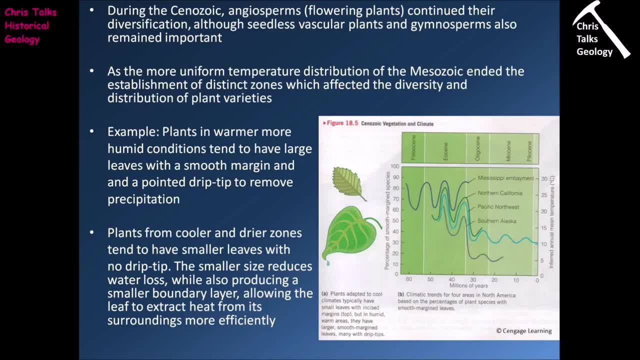 the more water you will lose through transpiration. now, if you're in a wet environment, like a rainforest, that's not a problem, because you can replenish the water. in contrast, when you are in a drier climatic band, well then you have a bit of an issue. so typically, the easiest thing to do is make 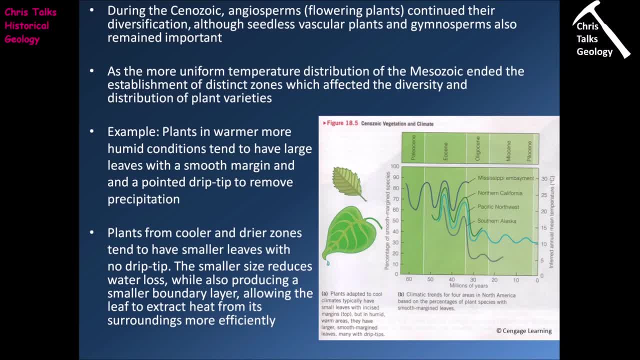 your leaves smaller to limit that water loss. now, the other change that the smaller leaf induces is a is a change in the thickness of the boundary layer. so the boundary layer is a layer of still air that surrounds the leaf. typically, the bigger the leaf, the thicker the boundary layer will be. 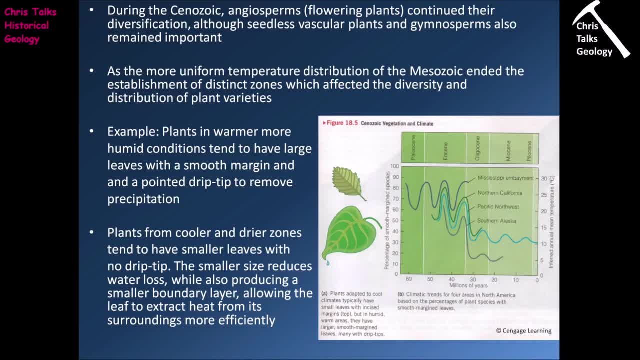 now the boundary layer is going to act as an insulator, so this means that if your leaf is on a plant in a hot, humid climate, it means that during the day, the leaf is going to get heated up and because the boundary layer is going to be quite thick, it means it's going to have difficulty. 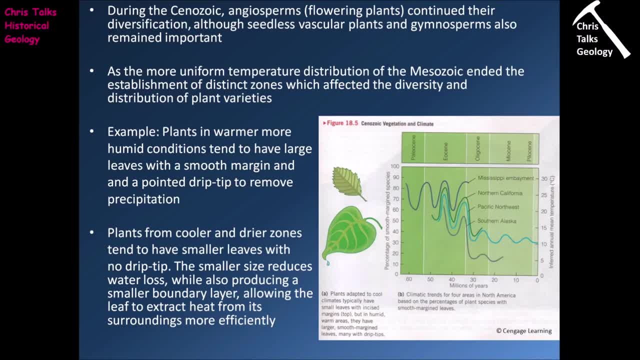 losing that heat, and so the only way the leaf can get rid of that excess heat is through transpiration. so by losing water. the boundary layer will then get even longer, and the impacted air will then be water. Now, this isn't a problem in humid climates. however, if you're in a drier climate, you can't. 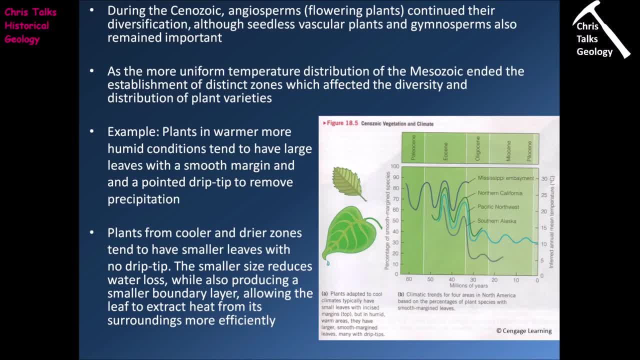 lose that water. so what you really want is a thin boundary layer so your leaf doesn't get too hot, and so having a smaller leaf allows you to have the thinner boundary layer, and this not only allows your heat to your leaf to not only overheat, it also allows your leaf to absorb heat from the. 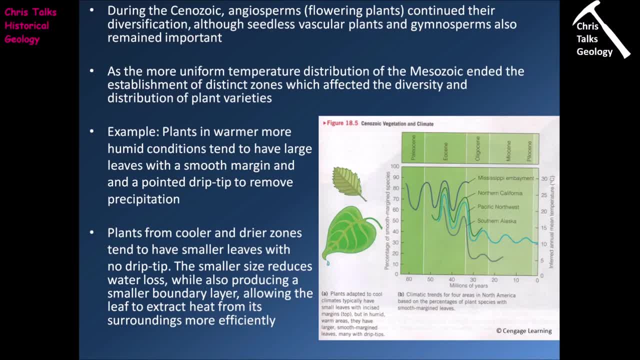 surrounding environment more efficiently, so this is going to reduce the chances of your leaf getting too cold and becoming damaged. So the diagram over here on the right is showing us changes in the percentage of plant species with smooth margin leaves from four locations in North America. So we have the Mississippi Embayment, Northern California, Pacific Northwest and 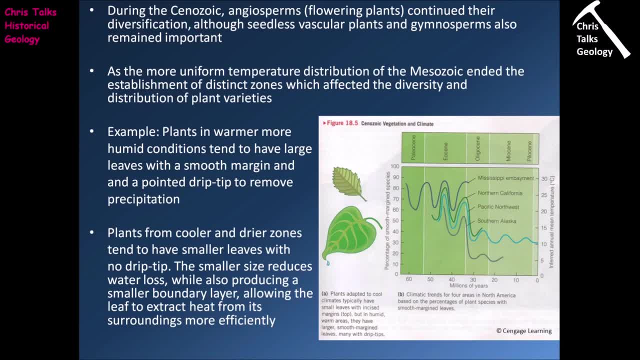 Southern Alaska. Now, we know that smooth margin leaves are associated with warm, humid conditions. so what you'll see is that for all of these four locations, we can see that a substantial portion of the flora in those areas during the Paleocene and the Eocene was made up of plants. 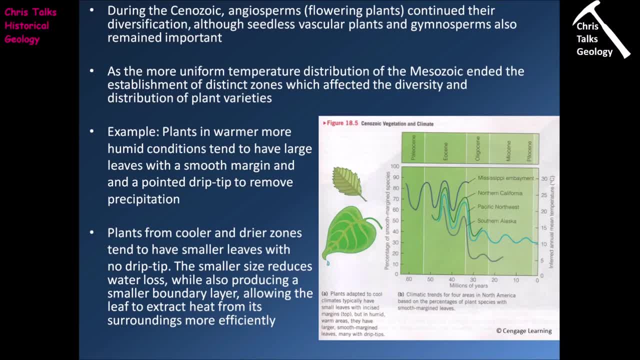 with smooth margin leaves. so this is telling us. conditions were, on the whole, quite warm and quite humid and of course, this makes perfect sense because we know that during the Paleocene and Eocene we were experiencing the high temperatures associated with the Paleocene Eocene thermal maximum. 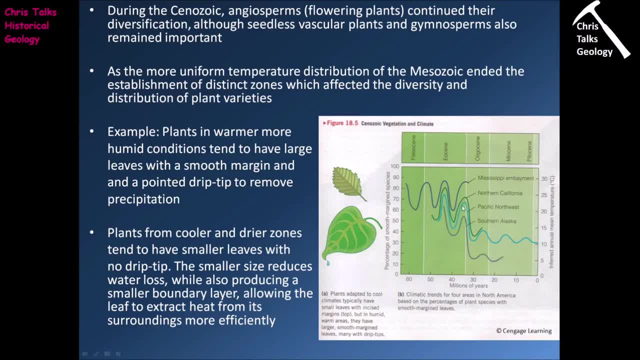 Now, as we move into the Oligocene, we can see that the percentage of smooth margin leaves in Northern California, the Pacific Northwest and Southern Alaska begins to drop off quite quickly. you can see it especially strongly there with the trend for Southern Alaska, and so this is showing. 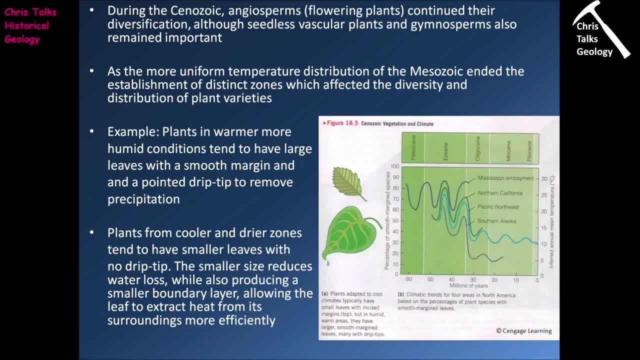 us that what we have is a situation where we are losing essentially these warm conditions, and conditions are getting colder and or drier. So we know that in the case of Northern California, it's going to stay relatively warm. however, things begin to get drier as we progress further into the 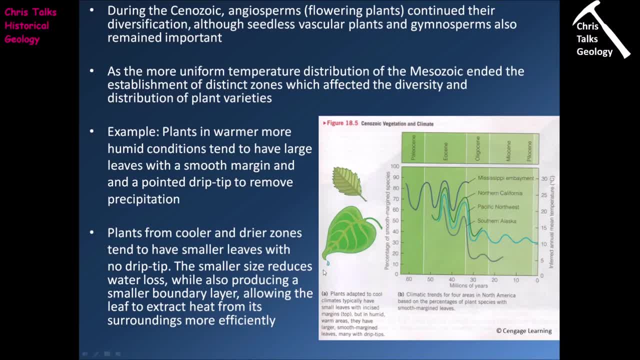 Cenozoic, so that's going to reduce the efficiency of the smooth margin leaves, and so we're going to see some plants that have smooth margin leaves beginning to become less common. In the case of the Pacific Northwest and Alaska, we have a decrease in temperature and so obviously this is going to 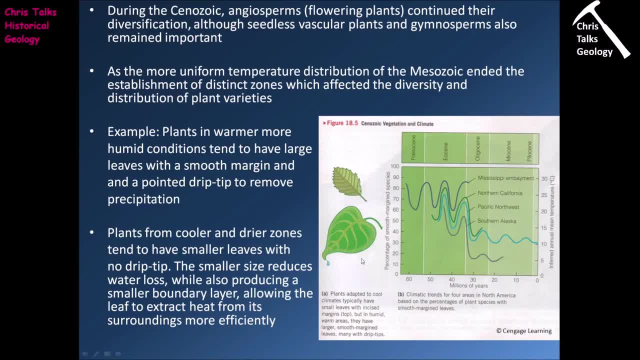 mean once again, having these big leaves is actually going to be a bit of a problem, and so you're going to see these large leafed plants being more and more common, and so we're going to see a lot of plants being replaced by plants that have smaller leaves, more suited to the colder conditions, and so 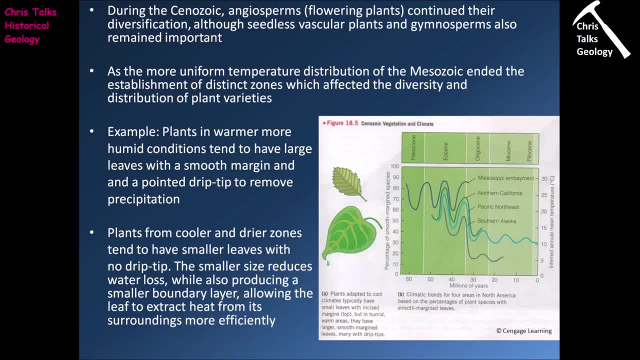 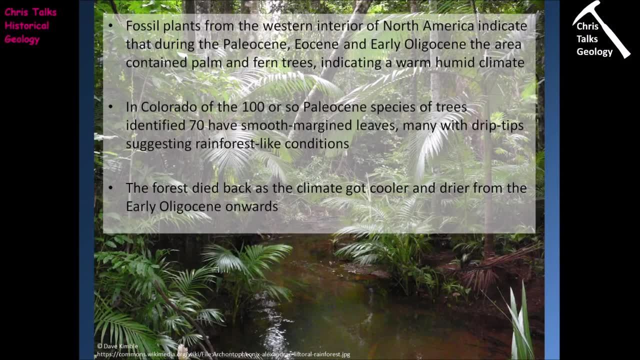 you know we can see this in the fossil record, and so this is a strong indicator showing us. you know, that we have this temperature change and we can see it from these plant fossils. Now, when we look at fossil plants from the western interior of North America, they indicate that 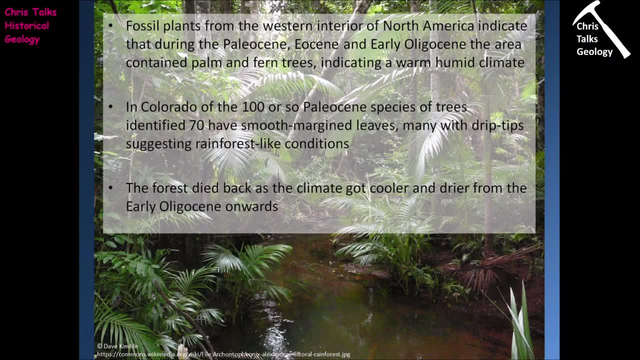 during the Paleocene, Eocene and earlier Ligocene. the area contained palms and fern trees, indicating humid climates. Now in Colorado, of the 100- or coincidence- species of trees identified, 70 of those had smooth margin leaves, many with drip tips, and that suggests leaves designed for a rainforest. 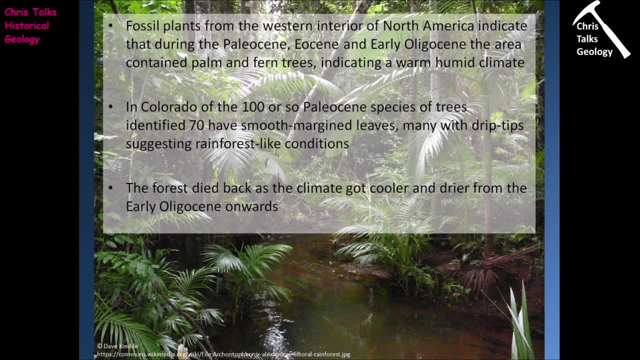 like set of conditions. so quite warm, quite humid. Now, as we transition into the Oligocene we begin to see these forests dying back as conditions get cooler and of course, as we've discussed, this is consistent with the gradual settlement of飯. at 10 1000mL ativae we can see leaf, ever Namka, wild orvan, as cold or as humid as can be, if both trees really are hot or just the forest becomes much warmer and soft, motor leichter, etc. 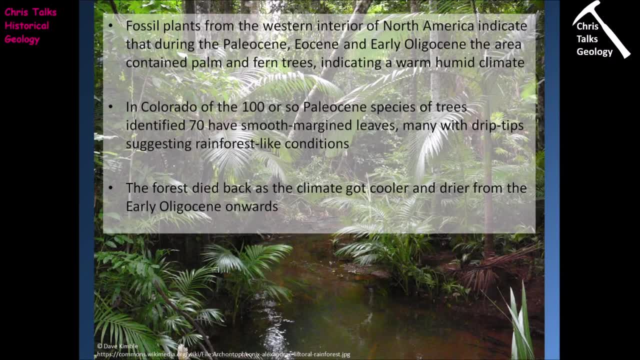 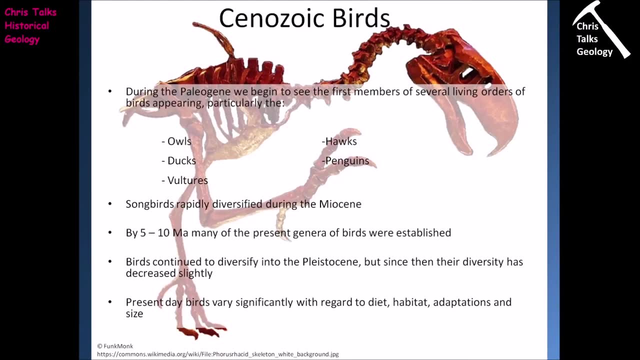 is consistent with the gradual temperature decrease which we see throughout the whole Cenozoic. So let's move on to Cenozoic vertebrates, and we're going to begin with Cenozoic birds. Now, during the Paleogene, we begin to see the first members of several living orders of 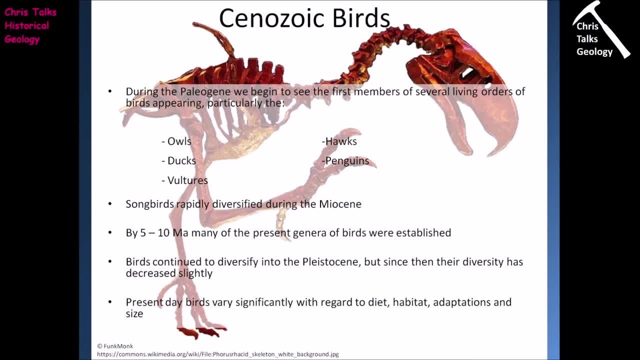 bird making their appearance. So we see orders like the owls, the ducks, the vultures, the hawks and the penguins beginning to appear. We see songbirds begin to diversify during the middle Cenozoic, particularly during the. 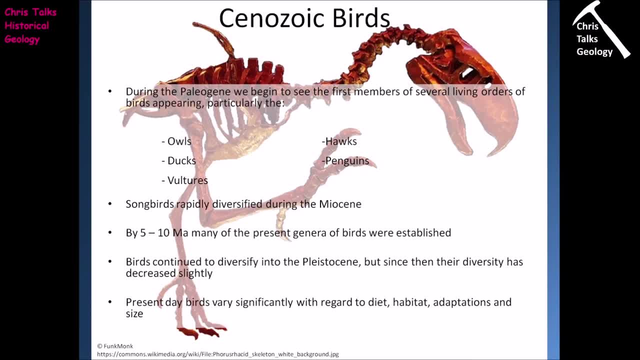 Miocene, and this means by about 5 to 10 million years ago, many of the present day genuses of birds were already established. So this means if we were to jump in a time machine and go back 7 million years. when we got out and we started looking at the birds which we saw, they would on the whole, look. 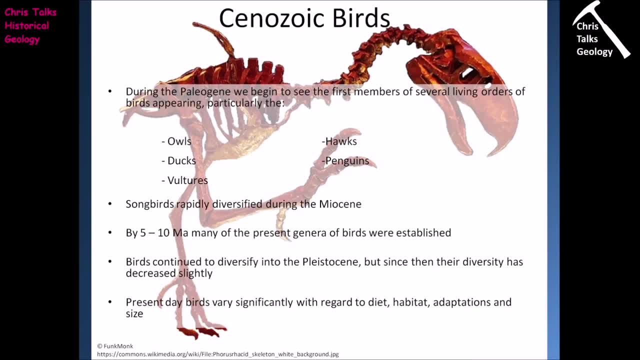 quite familiar to us. Now we see birds continue to diversify into the Pleistocene. however, from that point onwards, their diversity has decreased slightly. That's obviously going to be a reflection of the tougher conditions experienced during the Ice Age. Now, during the present day, we can see that birds vary significantly with regard to diet. 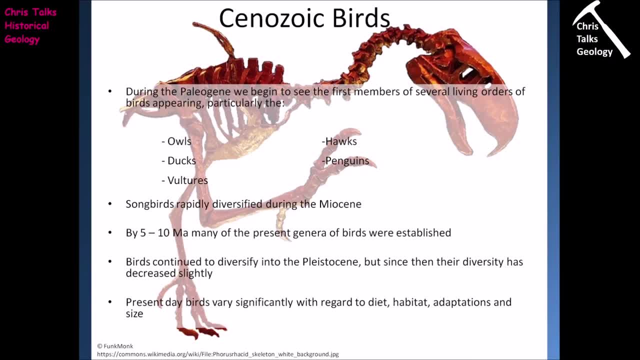 habitat adaptations and size, and this isn't a huge surprise because, of course, we know we have all these different climatic bands established during the Cenozoic. This obviously means that individual species of birds will have to adapt to their local environment, and so that's obviously going to lead to quite a lot of diversity in terms. 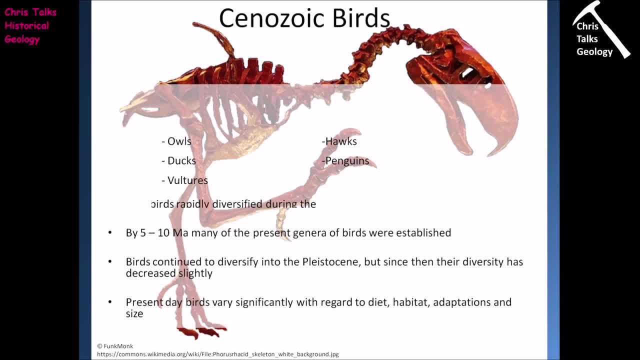 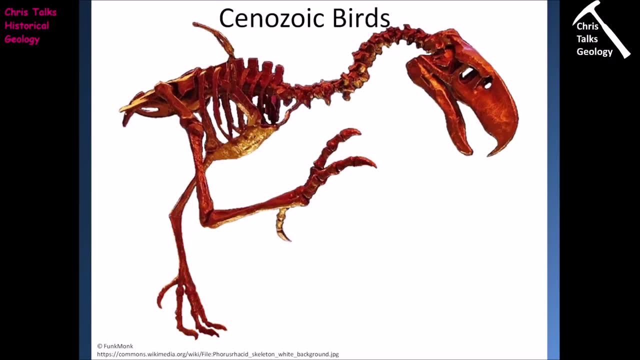 of body design. So just to give you some idea about some of the changes which we see when it comes to birds during the Cenozoic, the picture that we can see here is of a titanus bird, otherwise known as a pterobird, and they're going to become an interesting group that makes their 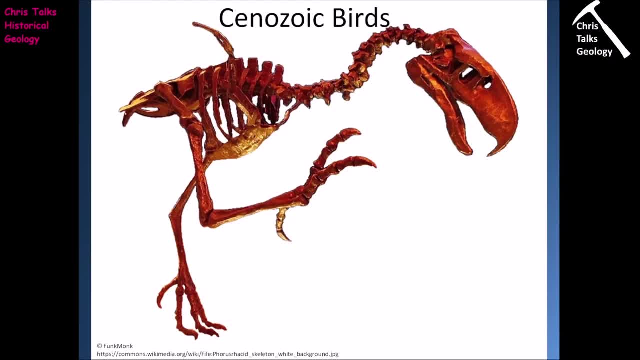 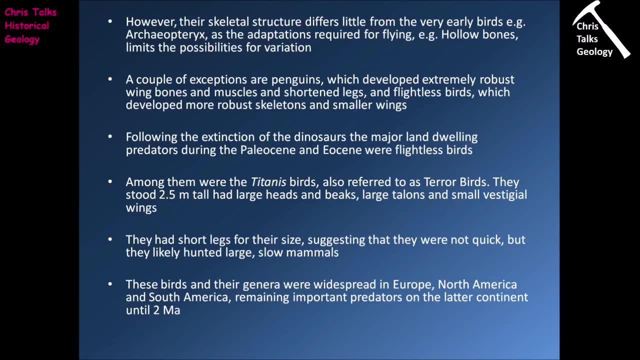 appearance during the Cenozoic, and we're actually going to discuss them in the next slide. When we look at the skeletal structures displayed by Cenozoic birds, we see they differ relatively little from the skeletal structures displayed by early birds from the Mesozoic. so something. 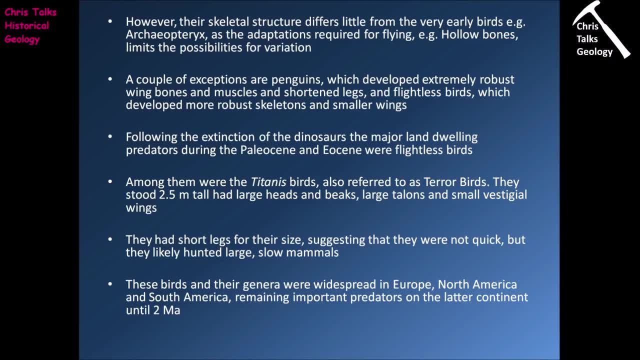 like Archaeopteryx. Now, this is because the adaptations required for things like flight- so hollow bones, for instance- really limit the possibility for variation, because once you've established a system that works, evolution isn't really going to change it that much. So, when it comes down to it, the birds that fly show relatively little variation in the 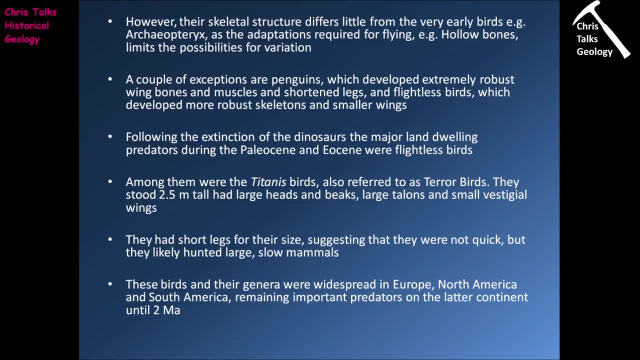 general design. Now, there are a couple of exceptions to this rule, and these are groups of birds that have developed to move into different environments, So the classic example would be the penguins. So the penguins have developed extremely robust wing bones and wing muscles, and they've also 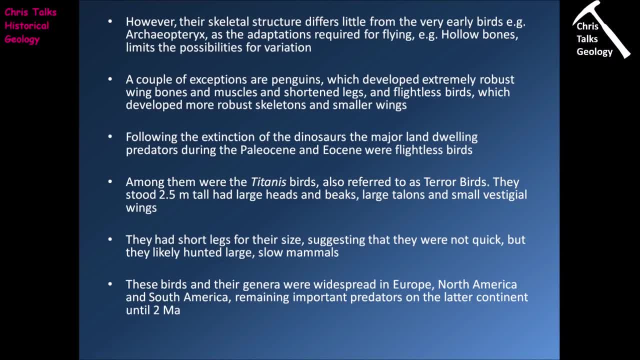 shortened their leg length, and this is a response of their movement into the marine environment. So obviously, the big, powerful wings are required for propulsion through the water, whilst the short legs help to create a more streamlined body In the case of the flightless birds. so let's, for instance, think of something like an ostrich. 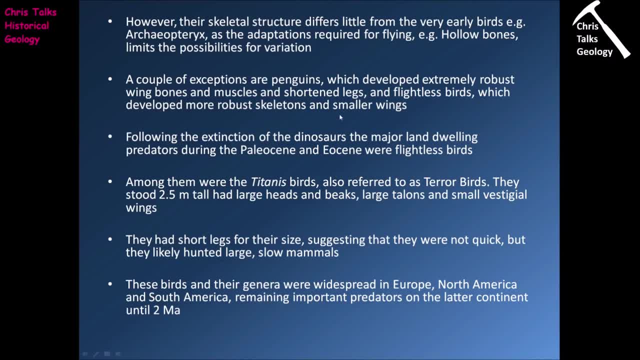 we see that they develop a more robust skeleton And they develop smaller wings. Typically, the smaller wings are because, well, if you're not flying, the wings will often actually get in the way. they're a bit of a hindrance. so having smaller wings can often 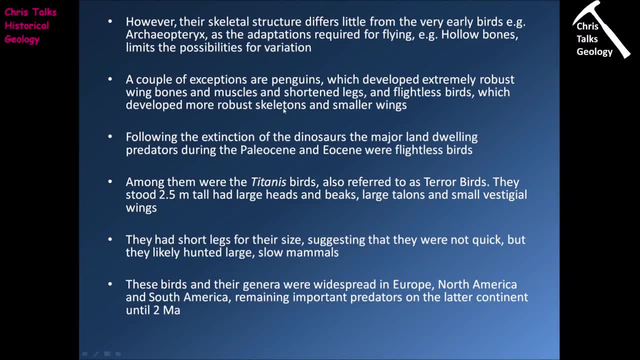 be advantageous In terms of the more robust skeletons. well, these are animals which are existing on the continents, so you know they don't have to worry themselves with having lighter bones designed for flight. So that means the bones can become bigger, more heavy set, stronger and obviously this: 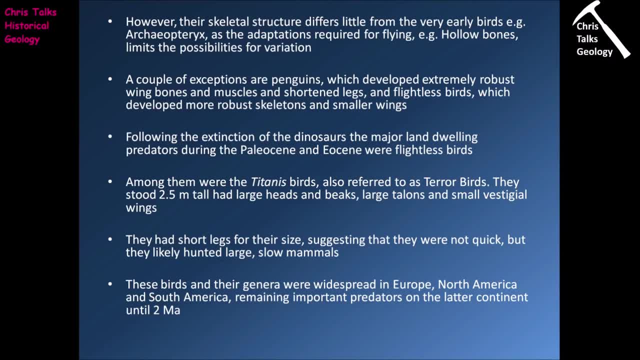 is going to be more advantageous for me Now. following the extinction of the dinosaurs, the major land dwelling predators during the Paleocene and Eocene were actually flightless birds. We typically assume that once the dinosaurs are gone, the mammals make their move and 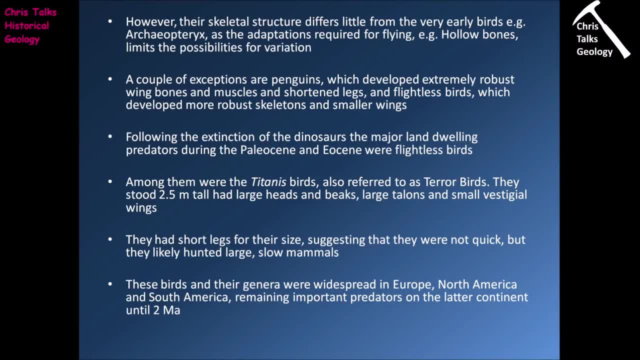 then that's pretty much it. In reality, though, it took a while for large mammalian predators to really become established, so the initial running was actually done by the flightless birds. Now, One of these Cenozoic birds, arguably the best known group, are the Titanus birds. 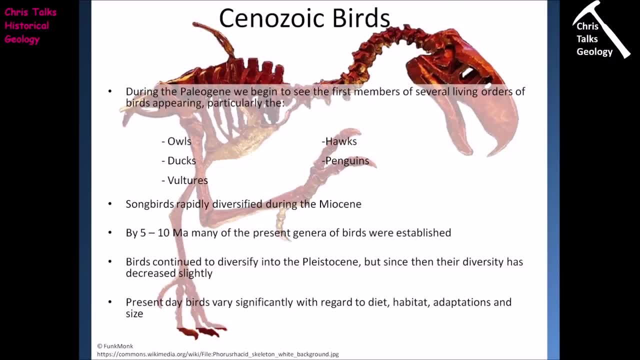 They are often referred to as the Terror birds and we saw a picture of one on the previous slide here. So you can see these birds have very big, very strong beaks designed for attacking their prey. They have strong, sturdy legs designed for movement on the continents, with long claws. 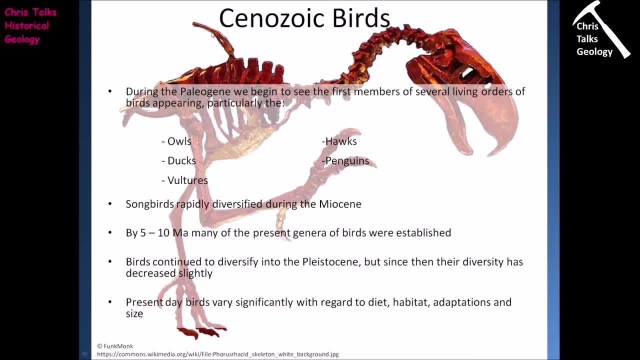 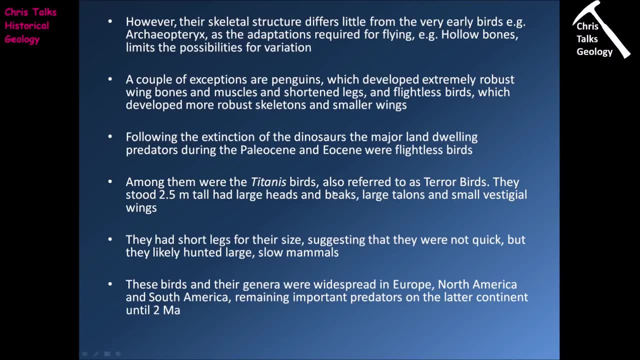 once again for attacking their prey, and we can see they have small vestigial wings. So, In terms of the Titanus bird design, they stood up to about two and a half meters in height at tallest. They had large heads with big, powerful beaks- as I say for attacking their prey, large talons. 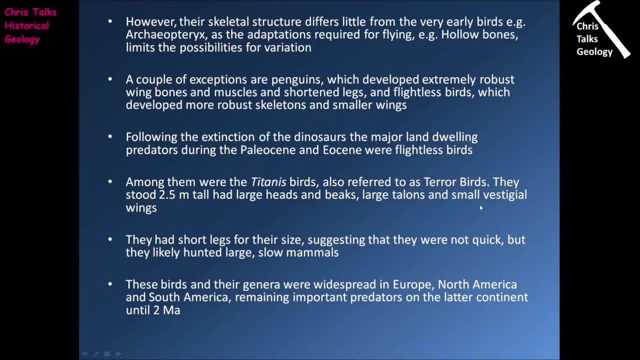 on their feet once again for attacking their prey and small vestigial wings. Now when we look at the Titanus bird design, we actually see for the size of them they had quite short legs. So if you think of something like an ostrich, we know that ostriches are quite quick and 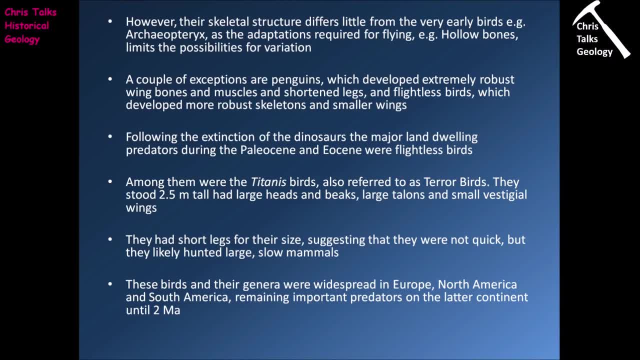 if we look at the ostrich, for the size of the bird, We can see it has very, very long legs. In comparison, the Titanus birds actually has shorter legs compared to its body size and this would suggest that, on the whole, the Titanus birds probably weren't that quick and they 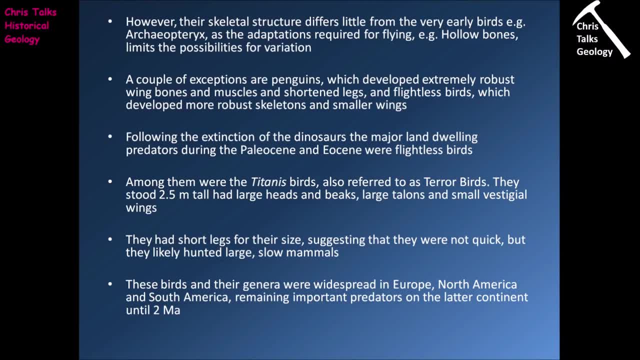 probably hunted larger, slower mammals as their prey, and this may well explain why their head design in particular becomes so amazingly overdeveloped, because, instead of you know going after smaller, faster prey, they're going after bigger, tougher prey. so you know, having really strong weapons Weaponry is going to be an advantage in terms of killing the animal you're going after. 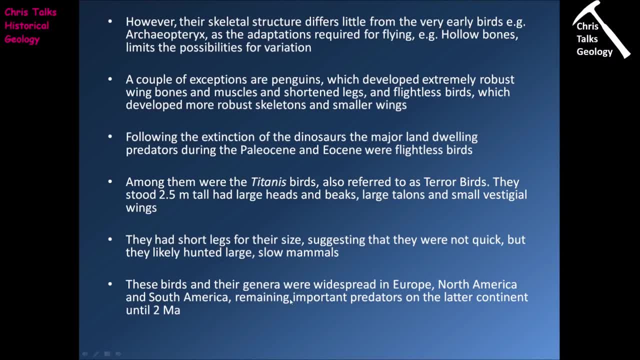 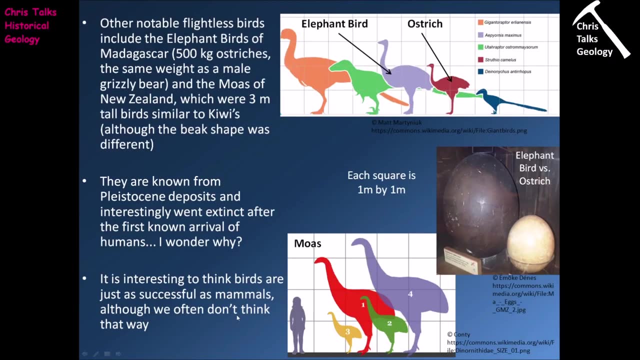 Now we see. the Titanus birds and their associated genus were widespread in Europe, North America and South America, and they remained important predators in South America up until about two million years ago Now. other noticeable flightless birds include the elephant birds of Madagascar. so just to 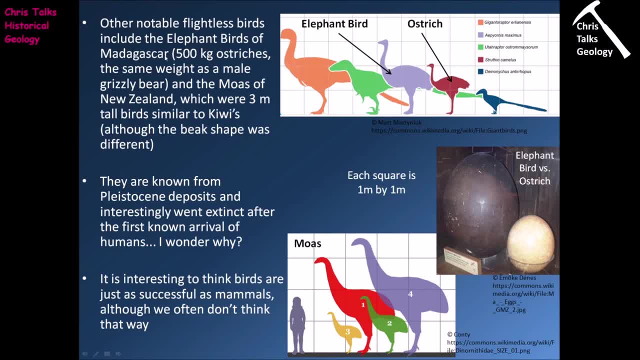 give you some idea, Titanus birds are about 500 kilograms in weight, which puts them at about the same mass as a male grizzly bear. so these were very big animals. and we also have the Nemoas of New Zealand, and they were three meter tall birds, similar to Kiwis, although the beak shape was